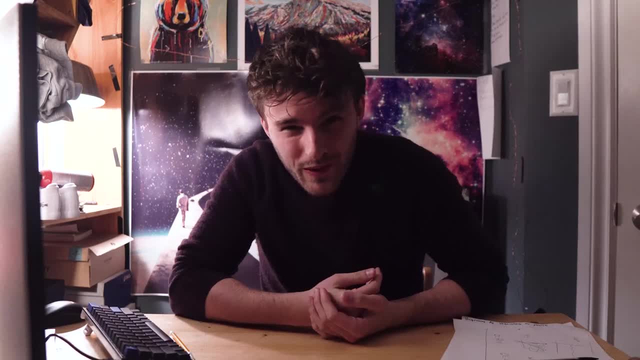 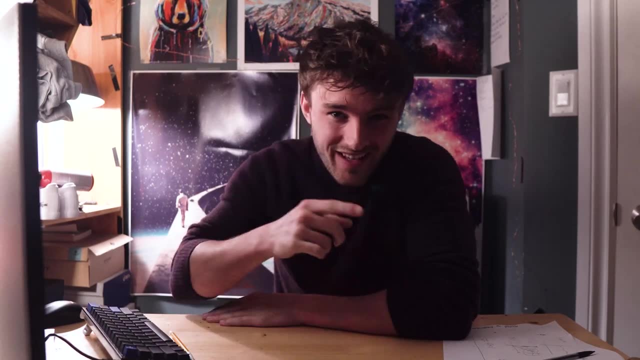 an insight I've had in the field. And then we're going to go to an old book by De Morgan, written in 1842, that I stumbled upon yesterday and I'm going to start reading A lot of old words in there. They spelt show as shoe S-H-O-W. They spelt S-H-E-W, 1842.. That's a long time. 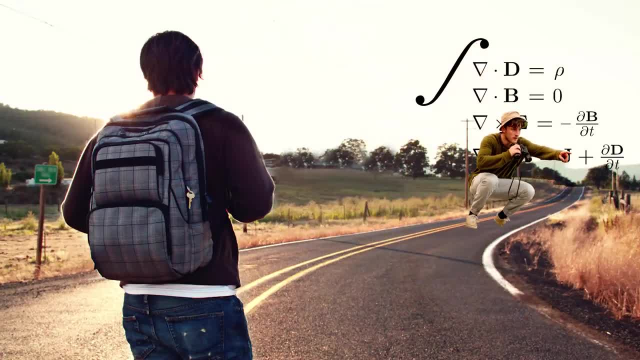 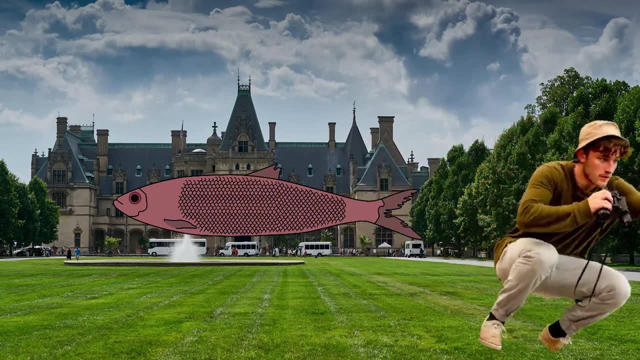 ago. All right, see you at the library. I am on a quest to understand and master high level mathematics. I tried university to get this done, but it wasn't the answer, And so I've left it to venture out on my own to find the knowledge I desire, Self-educating, using 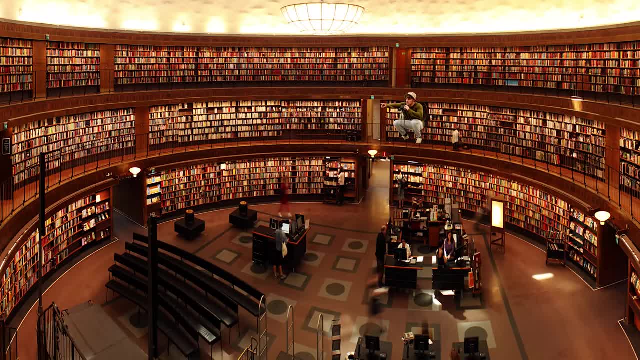 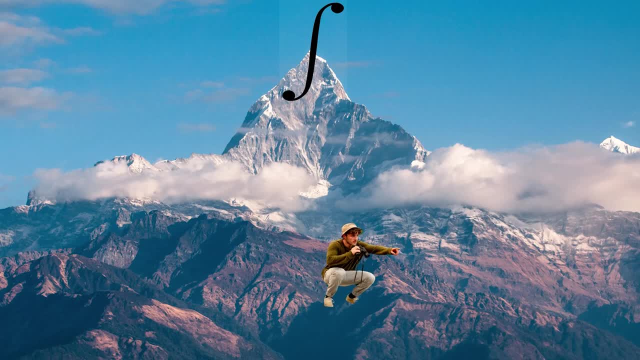 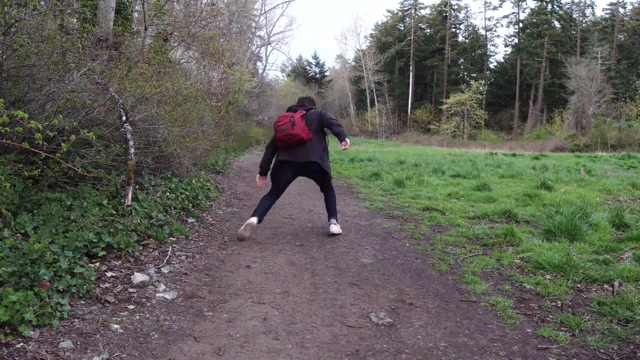 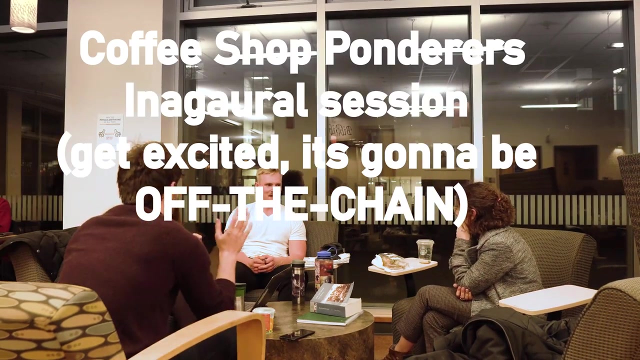 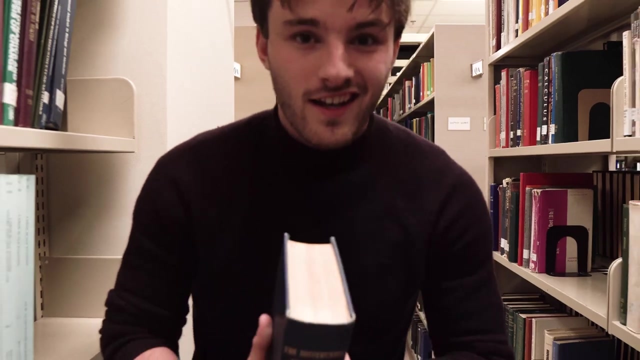 whatever resources I can find, documenting my journey as I go in order to help you in yours. The mountain is high and the path is long, So let's get to climbing. Okay, so yesterday I was looking for a book in calculus, more of like an older book on 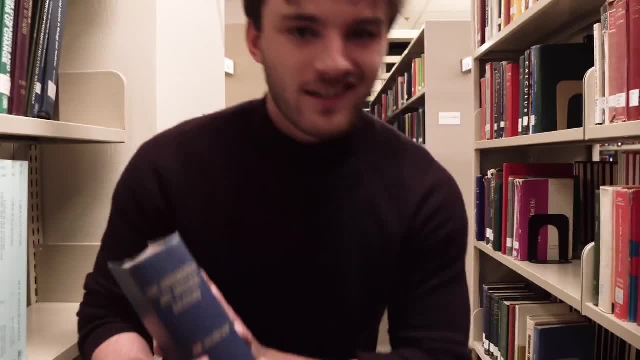 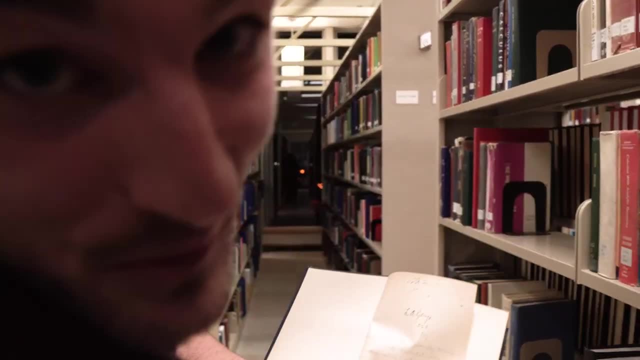 it And I saw De Morgan, which is a name I remembered from calculus class De Morgan's law, And I was like, oh, this is probably cool, Probably a reprint, I don't know if you can tell. Not a reprint. 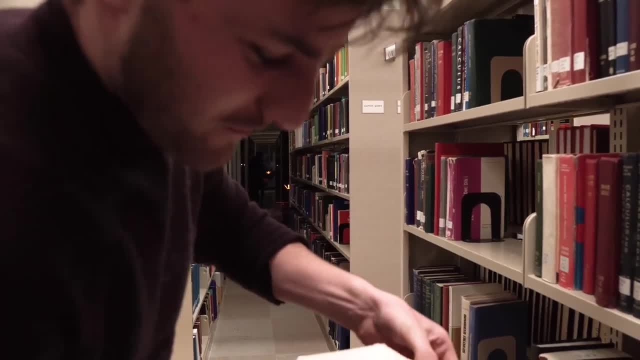 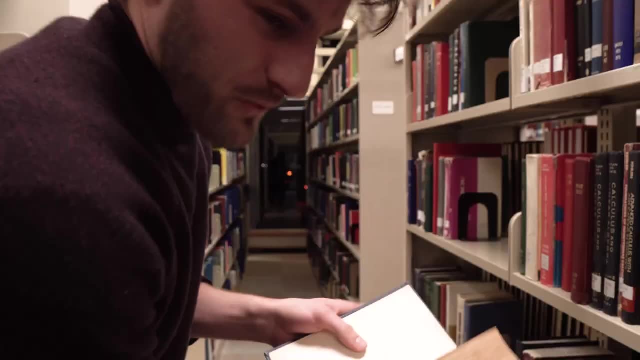 Literally, this is from like 18-something when this was written in there, I'm pretty sure. Look at that, Look at that handwriting. I don't even know where this book came from, but like ancient we're talking. 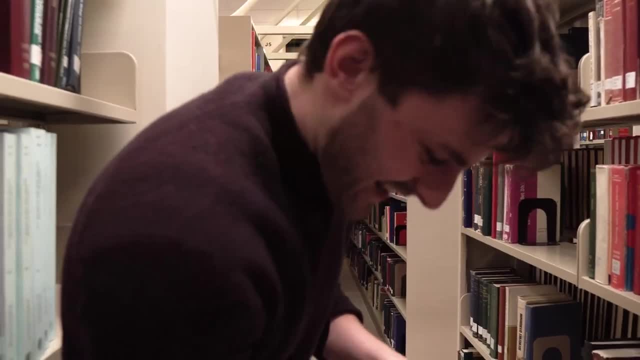 Written by literally De Morgan, Printed when De Morgan was still kicking. I was trying to find a date in it That says 1879-something. I think this was in a library of somewhere from 1879 to somewhere else. 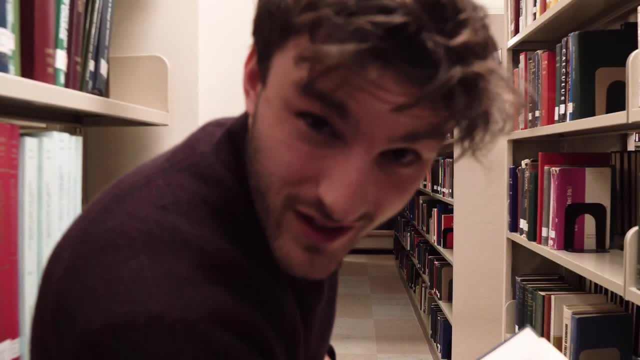 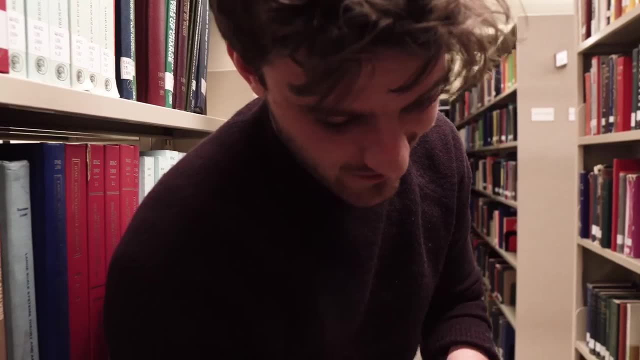 So I was looking through it, trying to find when it was printed, found the preface to the second edition, 1842.. It was printed in 1842.. I saw a handwritten quote in the beginning of it by Lord Kelvin. Oh, where's the quote? 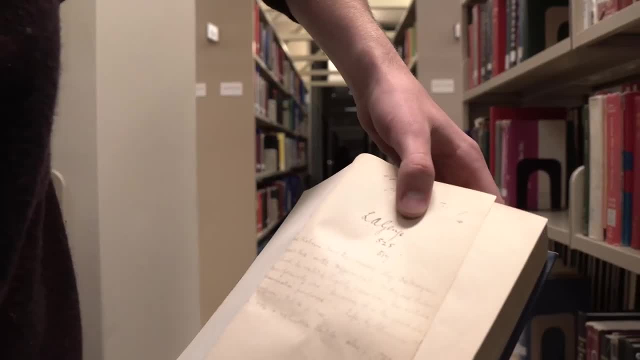 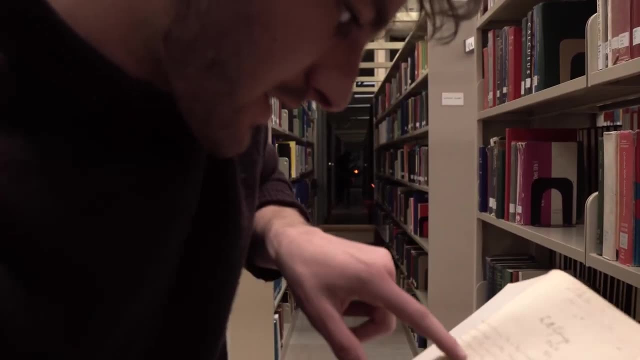 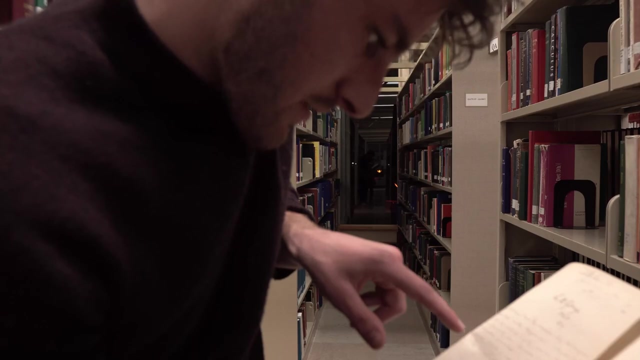 I don't know if you can read that Lord Kelvin said the reason why De Morgan's great book on the differential and integral calculus, which he valued highly, was now less valued than formerly was because it is too good for examination purposes. Life by somebody by Lord Kelvin. 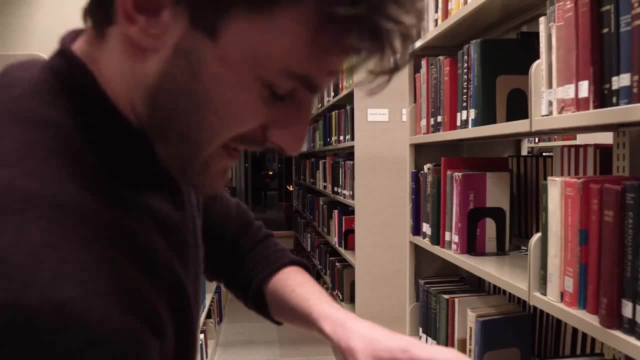 just a bunch of old books. So I took that book out of my bag and I'm going to go ahead. And then I'm going to read this book that I actually never read, which is very old. I've literally- this is from like 18 something, when this was written in there, I'm pretty sure. look. 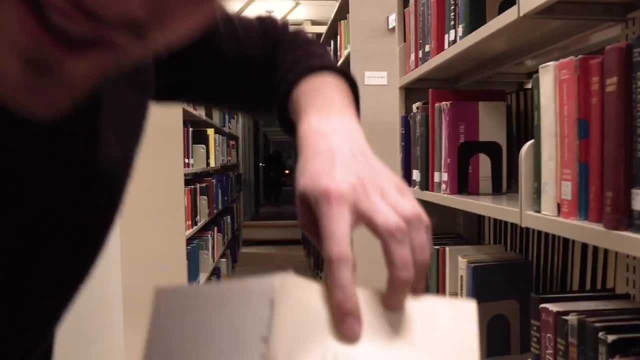 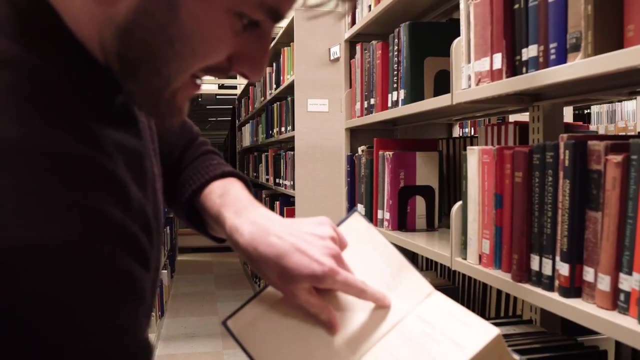 at that, look at that handwriting. I don't even know where this book came from, but like ancient, we're talking written by literally De Morgan, printed when De Morgan was still kicking. I was trying to find a date in it. okay, that says 1879 to something. I think this was in a library of. 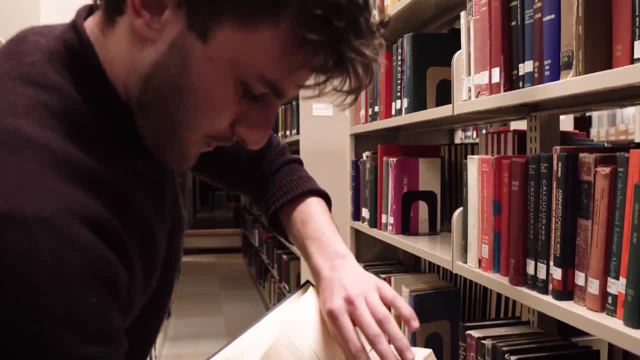 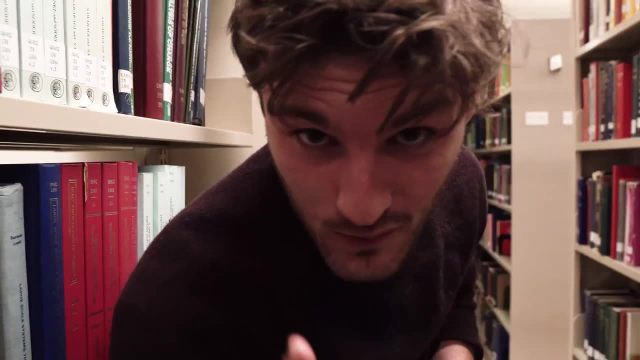 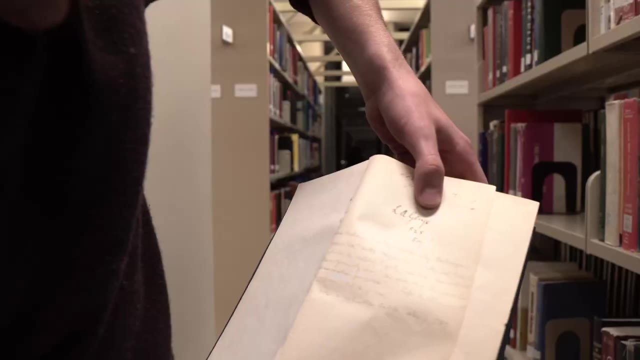 somewhere from 1879 to somewhere else. so I was looking through it trying to find when it was printed, found the preface to the second edition: 1842. it's printed 1842. I saw a handwritten quote in the beginning of it by Lord Kelvin. I don't know if you can read that. Lord Kelvin said the: 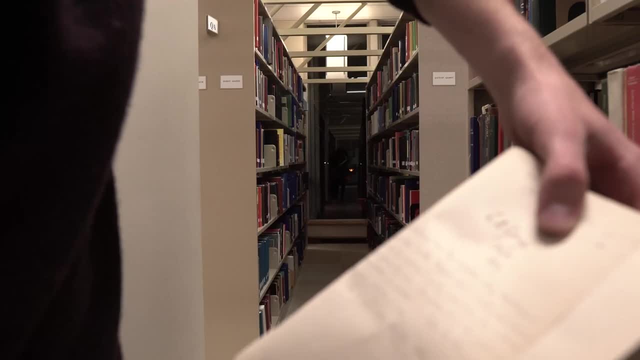 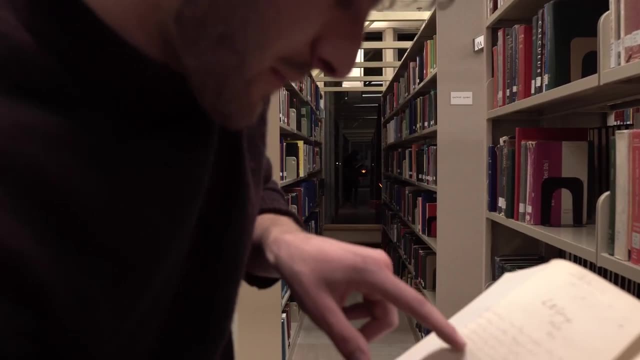 reason why De Morgan's great book of on the differential and integral calculus, which he valued highly, was now less valued than formerly was because it is too good for examination purposes. life by somebody about Lord Kelvin, so what needs to say? we got to read it because that's. 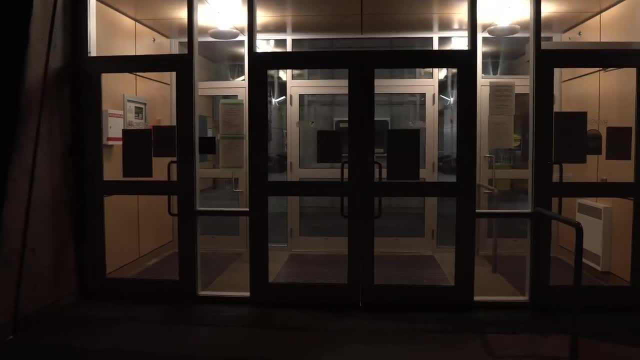 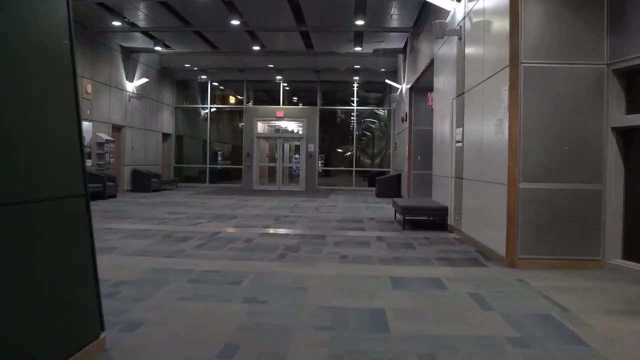 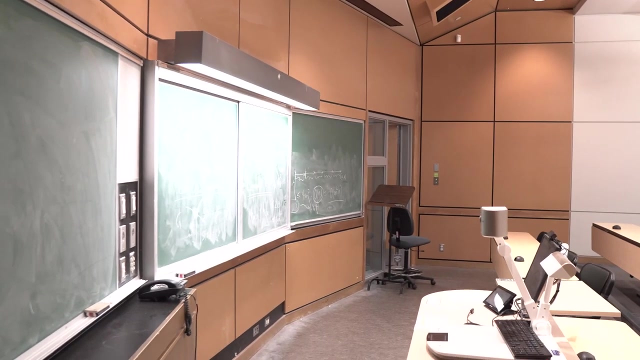 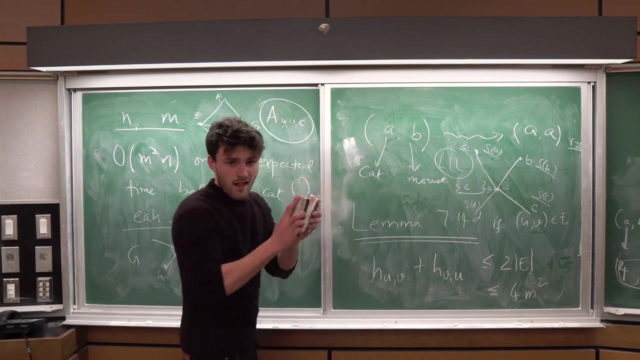 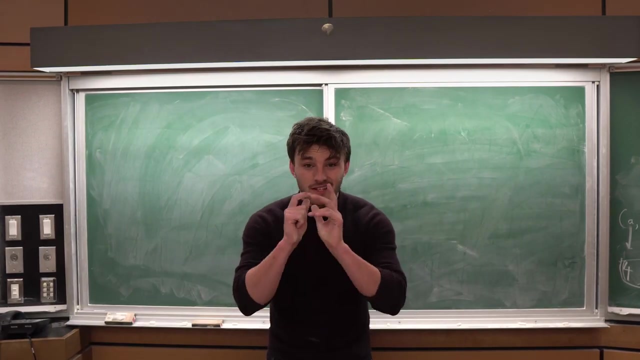 just absolutely goaded presentation time, so I'm going to give a fictitious yet pertinent approach to how matrices were invented. it was a very important approach to how matrices were invented, so I'm going to give a fictitious yet pertinent approach to how matrices were invented. 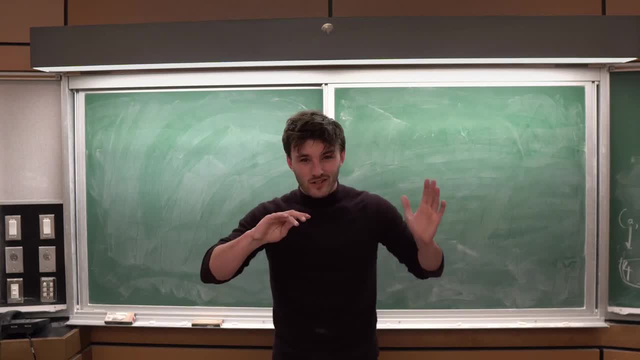 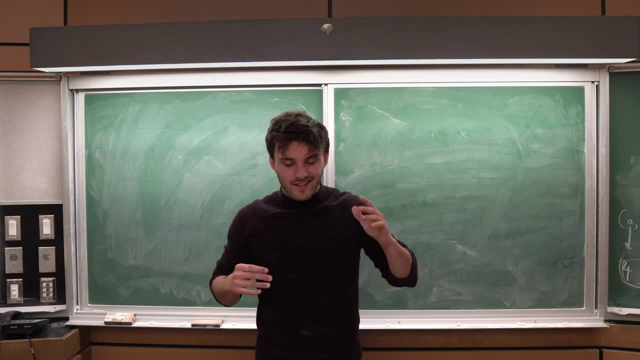 works logically. it's not how they actually came about. it might be. I haven't looked at the whole history, but I found this a useful heuristic for learning. mathematics is kind of make up some hypothetical history that's logically based, and then when you go back and learn the actual history, 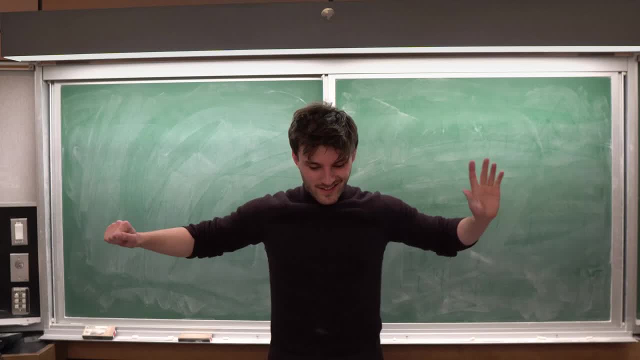 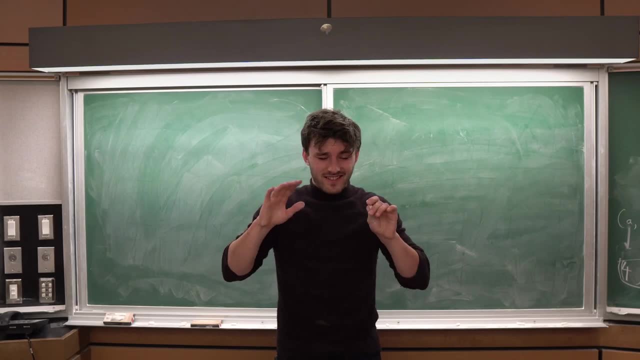 of a topic. in math it's like way more of a pain in the ass. like usually, some genius came along and then everybody's operating here and then they went like how about this thing? and then it makes absolutely no sense because they're like just stupidly smart and so the plebs have to come. 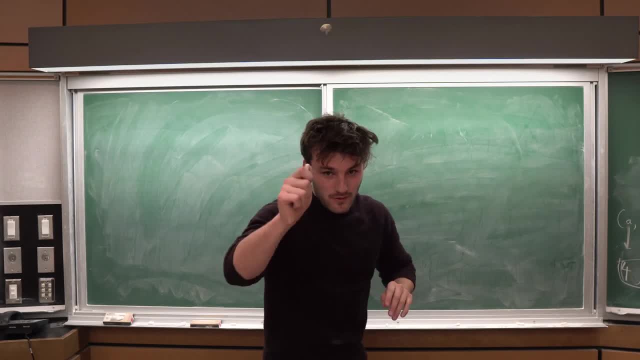 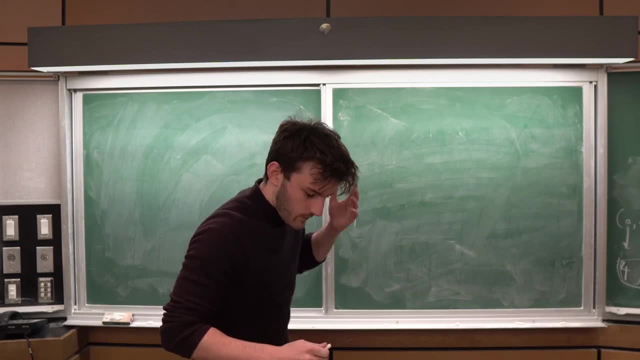 along like us later and then figure it out. but there is usually a logical step to take, and that's I'm gonna give here. we're talking about matrices and what they actually are. I never understood this. I've taken a lot of linear algebra but never understood what we were doing. matrices understood. 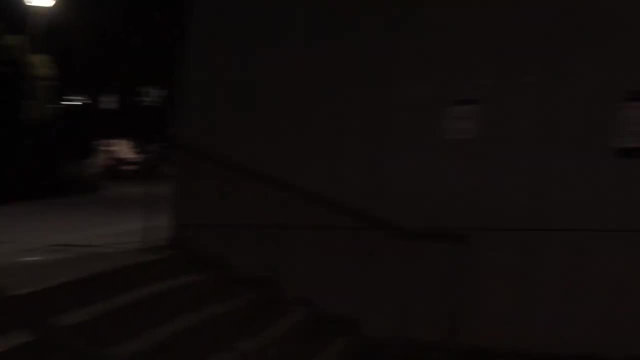 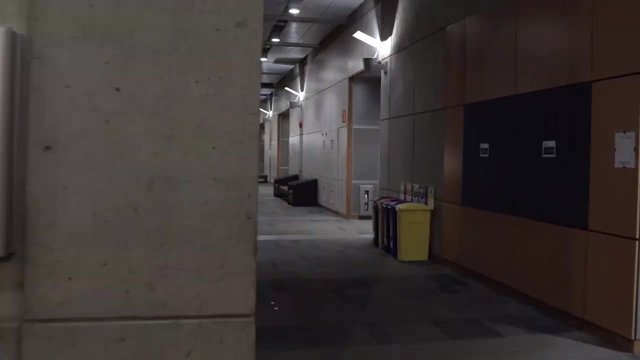 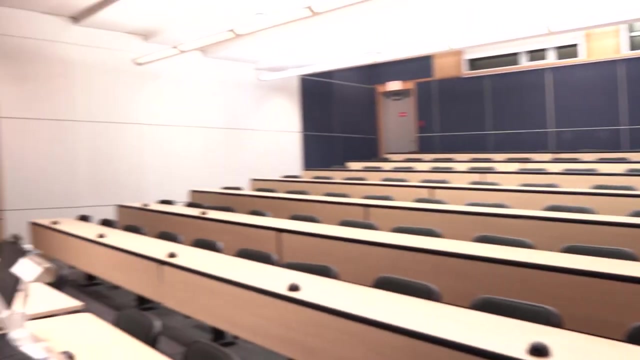 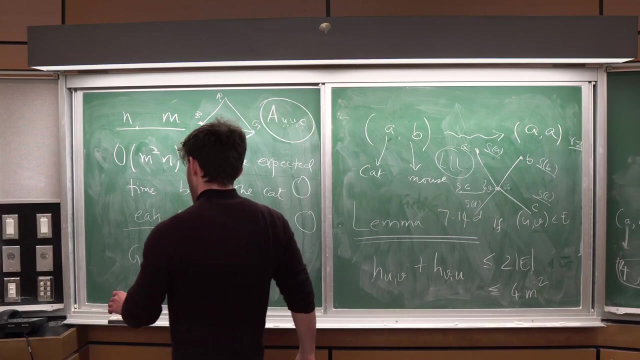 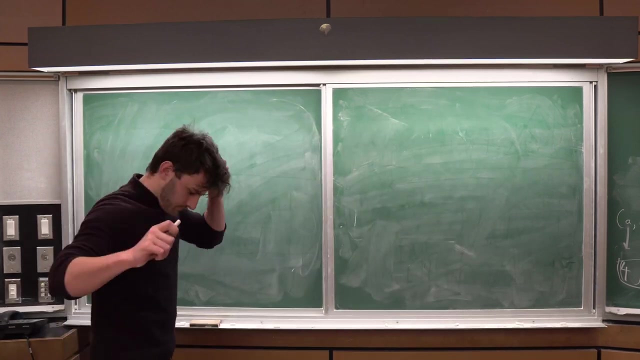 So what needs to say? we got to read it because that's just absolutely goaded Presentation time. So I'm going to give a fictitious yet pertinent approach to how a matrix should be handled To make a good book. So let's go ahead and get into it. 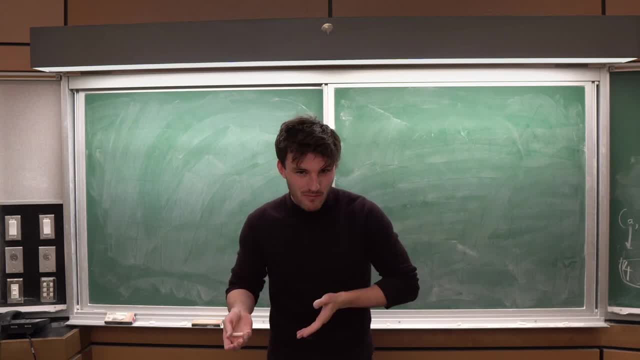 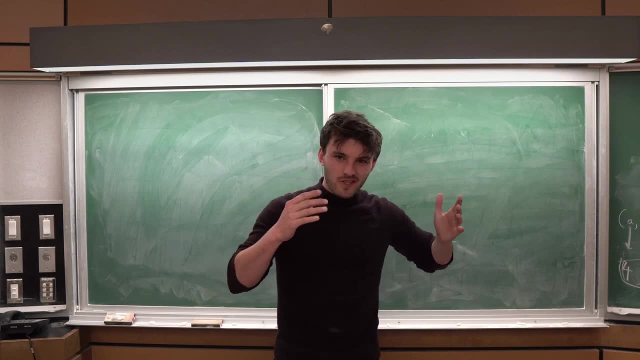 were invented. It works logically. It's not how they actually came about. It might be. I haven't looked at the whole history, but I found this a useful heuristic for learning. mathematics is kind of make up some hypothetical history that's logically based. And then when you go back and 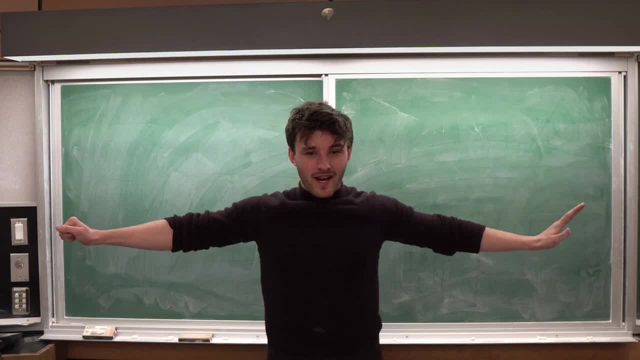 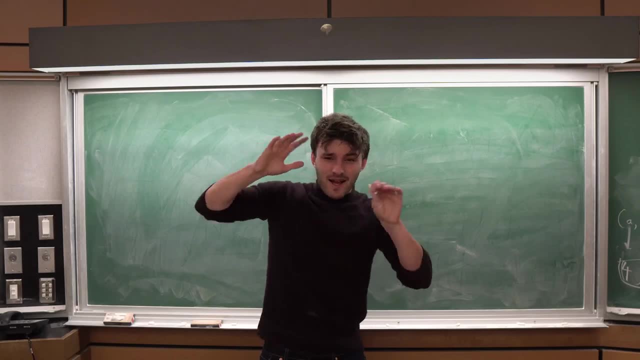 learn the actual history of a topic in math. it's like way more pain in the ass, Like usually. some genius came along and then everybody's operating here And then they went like how about this thing? And then it makes absolutely no sense, Cause they're like just stupidly smart And so. 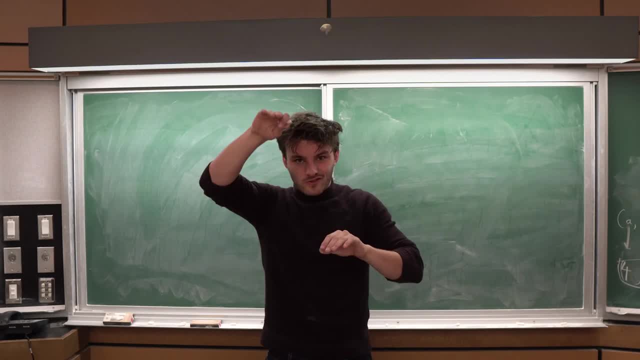 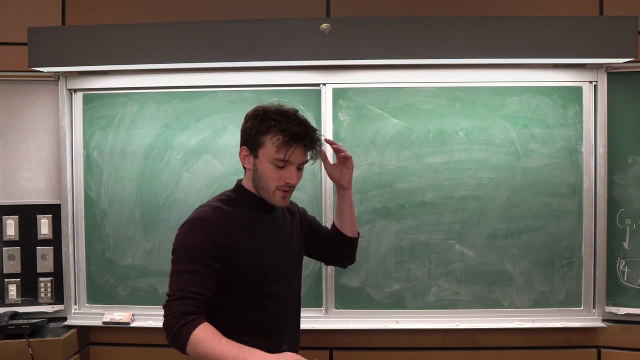 the plans have to come along, like us later and then figure it out. But there is usually a logical step to take And that's what I'm gonna give here. We're talking about matrices and what they actually are. I never understood this. I've taken a lot of linear algebra but never understood what. 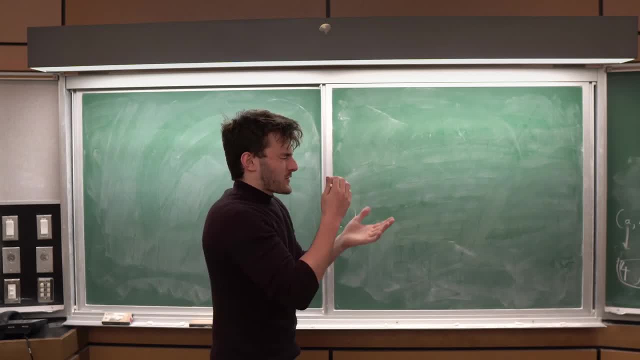 we were doing, Matrices understood the rules of manipulation, but what they actually were doing, how to think of them, totally had no idea. And so after a lot of digging it turns out that they're actually like pretty simple, uh, how they evolved, And there's a few logical steps you can. 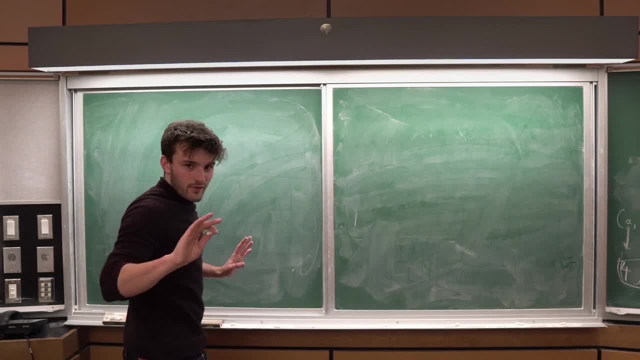 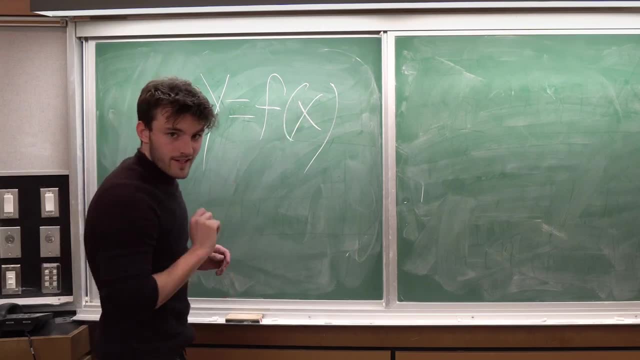 take to get there. So I'm gonna take you back, starting with the function. If you're watching this, you probably know what a function is: Single variable. five was F of S. you know one number goes in, one number comes out: Bob's, your uncle. 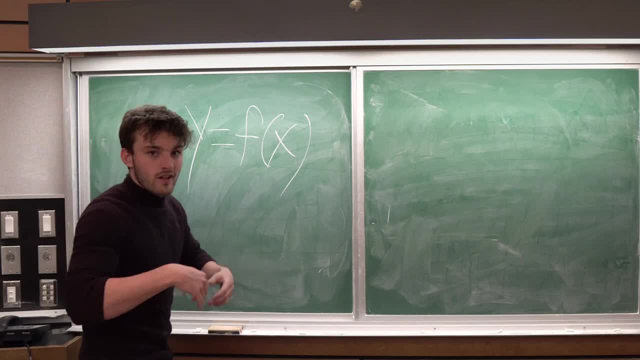 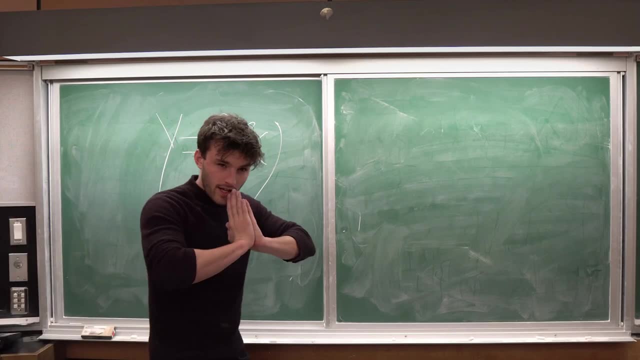 So you can think of it like a machine that takes in numbers and spits out numbers. There we go, And then this evolves over time. You know, some application comes along and he's like: all right, okay, I see you. I see you. one in, one out, Why don't we? why don't we? I don't know. 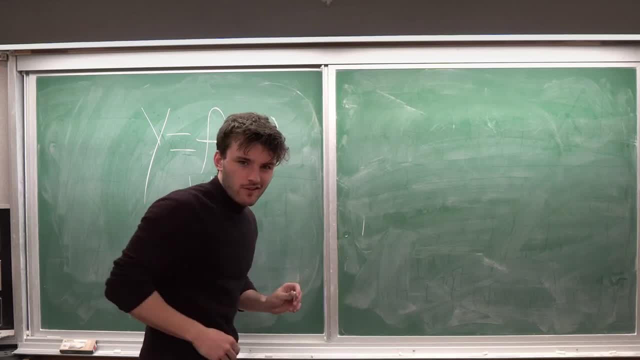 send two numbers in. Why don't we send two numbers in and see what happens? Two numbers in, one number out And everyone's like I don't know dude. that's kind of- I mean kind of- crazy dude, Like functions are. 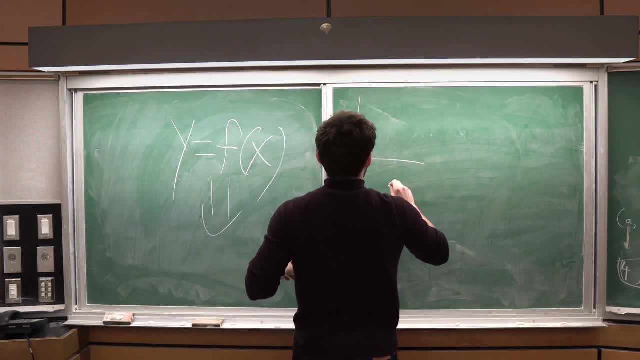 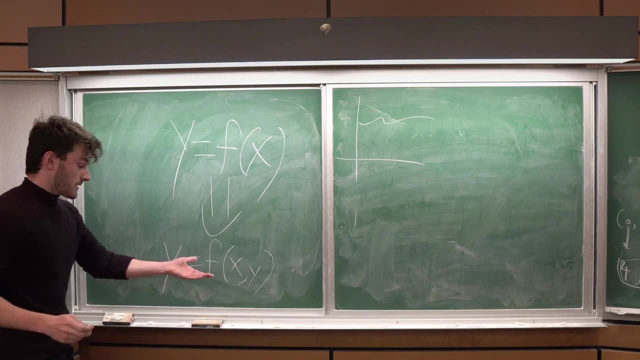 working with the Cartesian. you know we were doing, they were doing a doing this thing that's represented, and you have functions that's one dimensional. you know what? what even is a two dimensional function And, uh, this was a big, probably a big leap, Maybe I don't know, Uh, 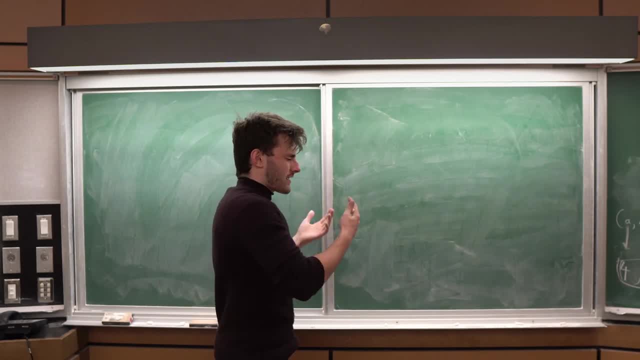 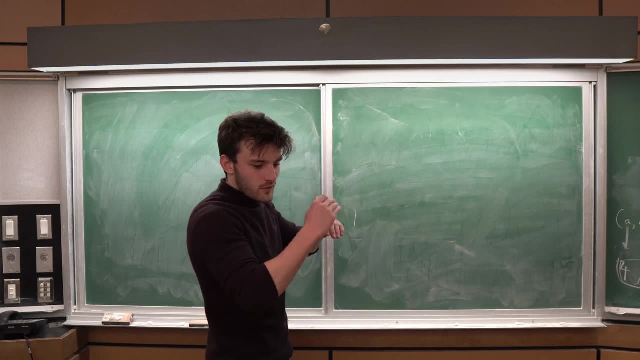 the rules of manipulation, but what they actually were doing, how to think of them, totally had no idea, and so, after a lot of digging, it turns out that are actually like pretty simple how they evolved, and there's a few logical steps you take to get there. so let's take you back, starting with 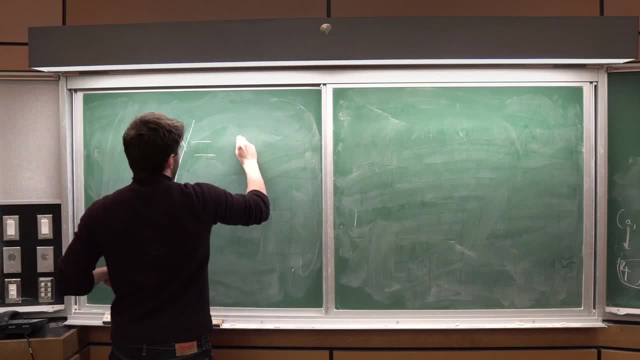 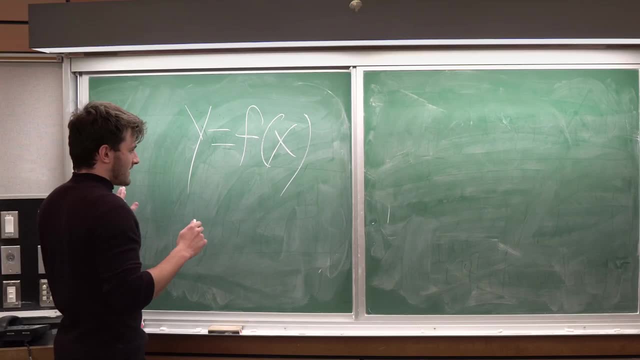 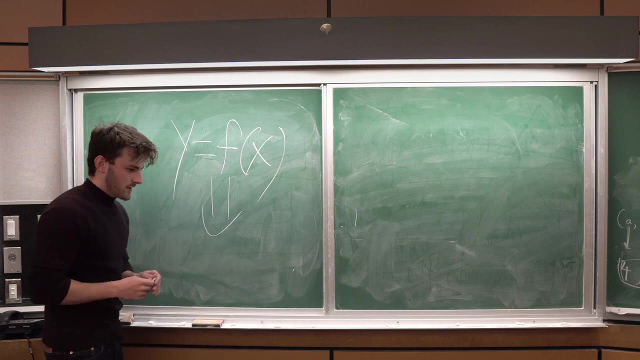 the function. if you're watching this probably know the function is single variable. why was that? the best you know, one number goes in, one number comes out. Bob, your uncle, you think of it like machine that takes in numbers and spits out numbers. there we go, and then this evolves over time. you know, some application comes along. he's. 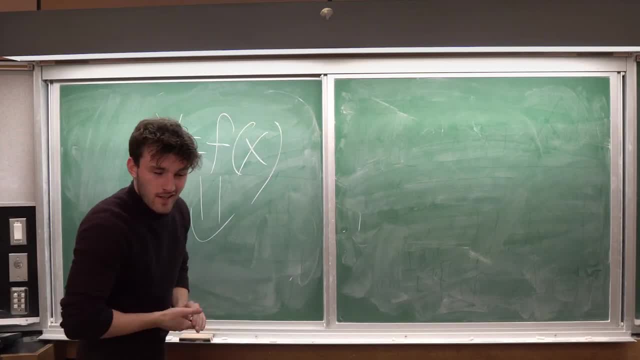 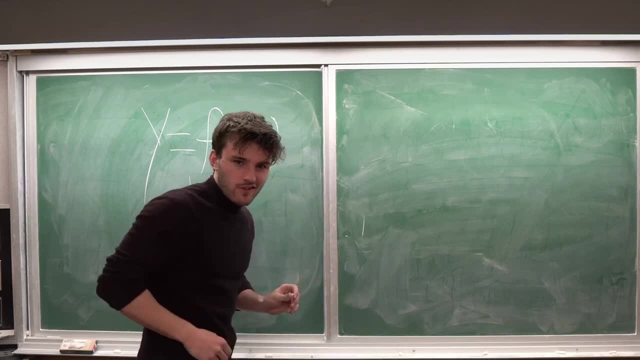 like: all right, okay, I see you, I see you one in, one out. why don't we, why don't we- I don't know- send two numbers in? when we sent two numbers in, see what happens: two numbers in, one number out, and everyone's like I don't know. dude, that's kind of- I mean kind of- crazy dude, like functions are. 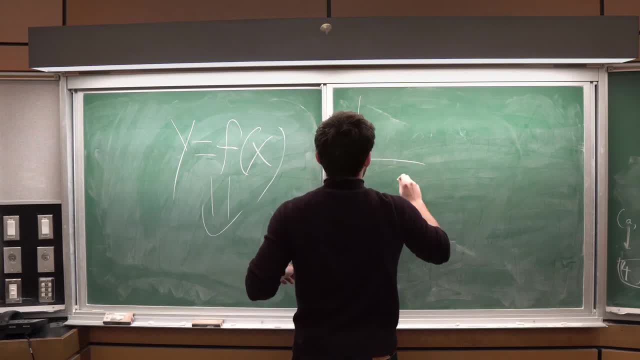 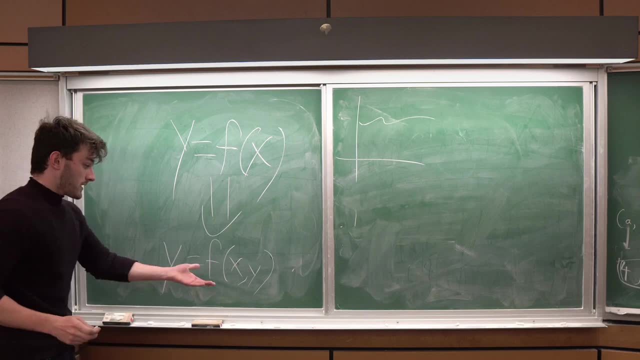 working with the Cartesian, you know we were doing, they were doing this thing that's represented and functions that's one dimensional. you know what? what even is a two-dimensional function? and uh, this is a big, probably a big leaf, maybe I don't know. uh, two numbers in one number out, that's that's. 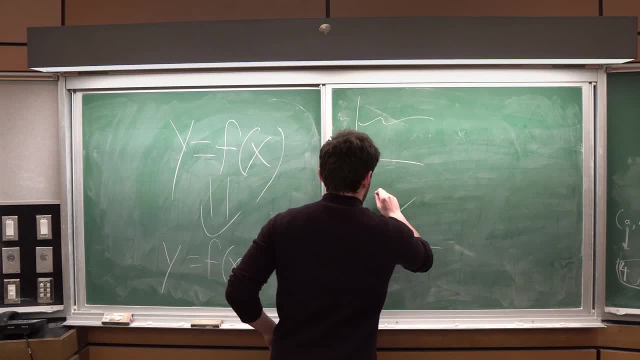 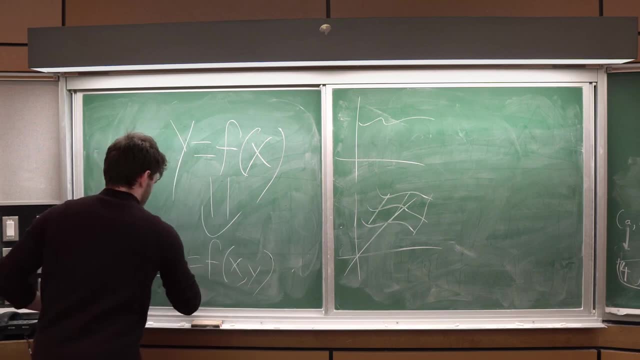 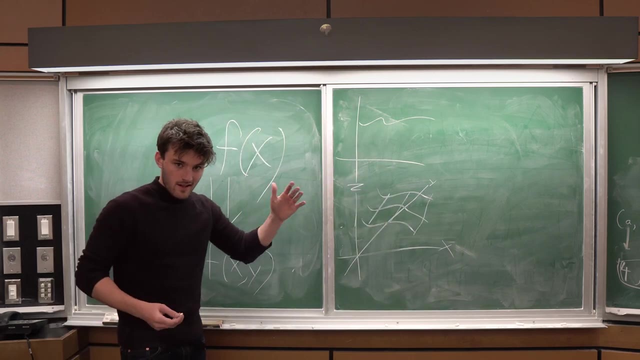 the the function box now, and you probably know what it represents. it's you're, you're or something like that. so it's a. you know the height, that's better. so this is the XYZ, and then represented as, like height is represented by where you are on the plane, and so that's all well and good. then somebody else. 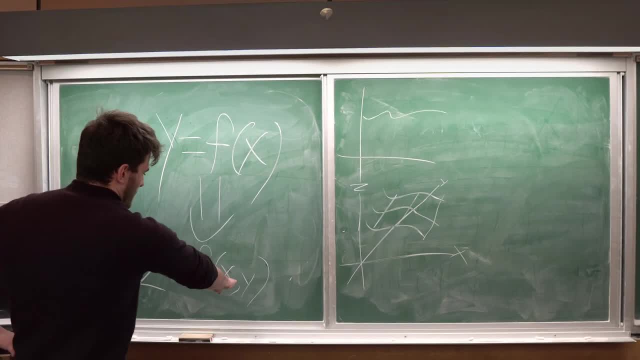 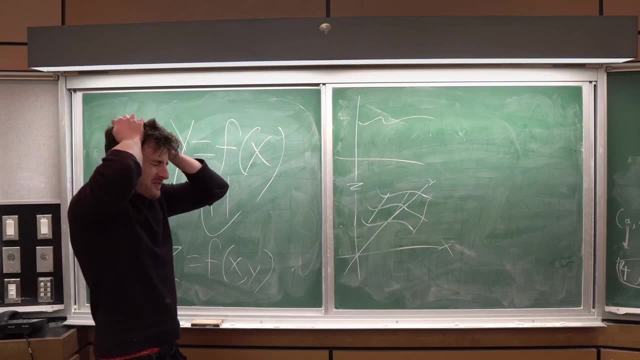 comes along and he says: why don't we just make it n-dimensional? why don't we have like 45 inputs to one output and, uh, everyone's like: dude, that's crazy, you're crazy, dog, you're wild and out bro. what are you talking about? how? how are we going to represent? like we have three dimensions? that's. 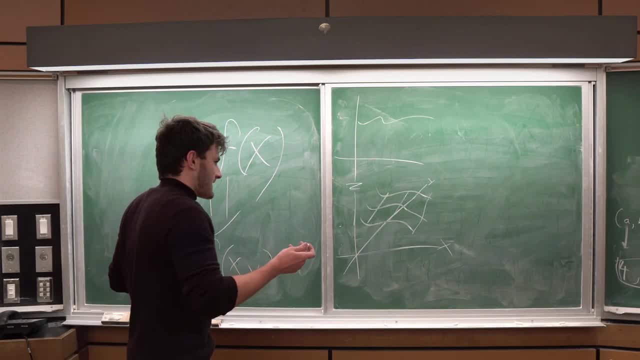 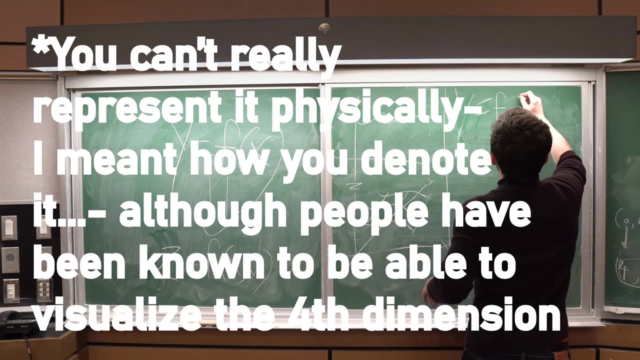 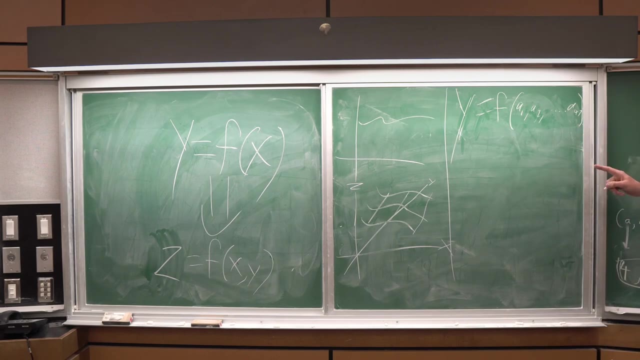 like a 45 dimensional function. what are you talking about? um? and so you represent that like, I don't know, like Y equals F, of something like that, and they still have, at the end of the day, you still have one output number. there's one number being output, a bunch of numbers being input. so then some absolute madman, some bad. 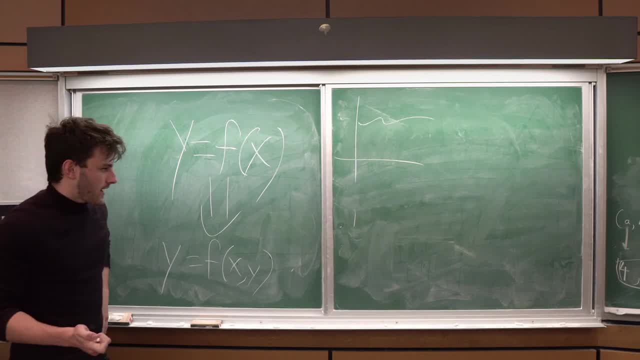 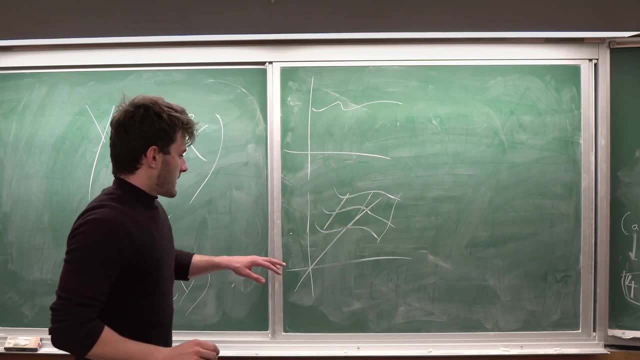 two numbers in one number out, That's. that's the, the function box now, And you probably know what it represented. This is your, your, your or something like that. So it's- uh, you know the height? that's better. So this is the. 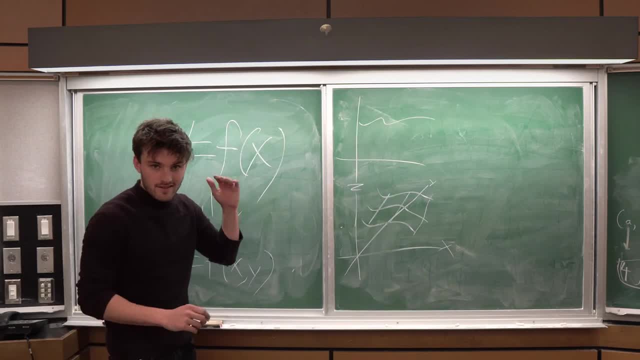 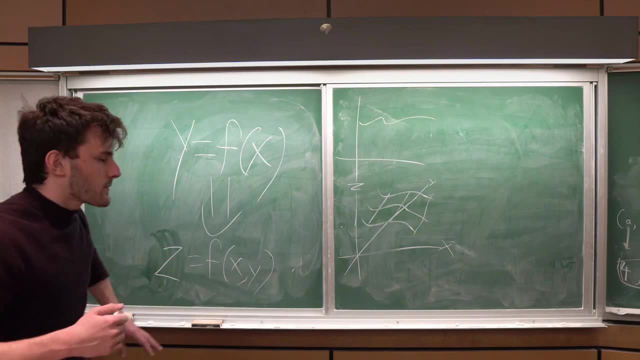 X, Y, Z and then represented as like. height is determined by where you are on the plane, And so that's all well and good. Then somebody else comes along and he says: why don't we just make it n-dimensional? Why don't we have like 45 inputs to one output? And uh, everyone's like dude. 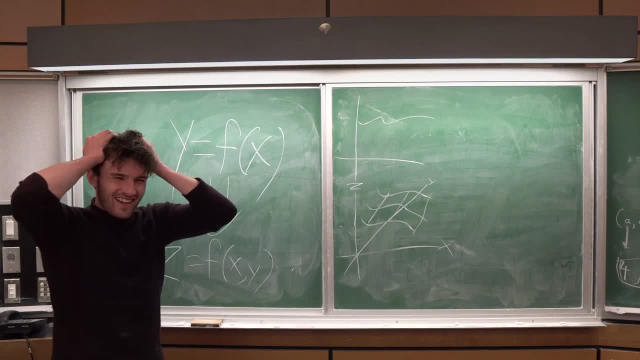 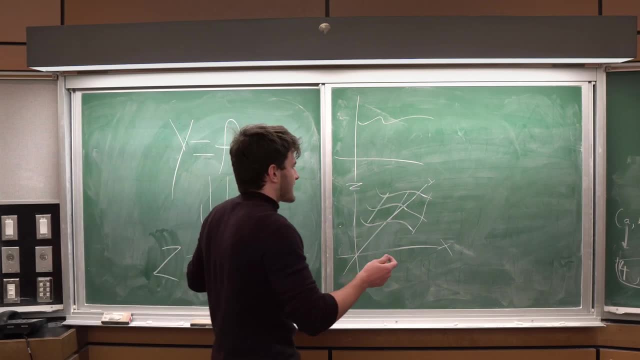 that's crazy. You're crazy dog, You're wild and out bro. What are you talking about? How? how are we going to represent, like, we have three dimensions, That's like a 45 dimensional function. What are you talking about? Um, and so you represent that like. 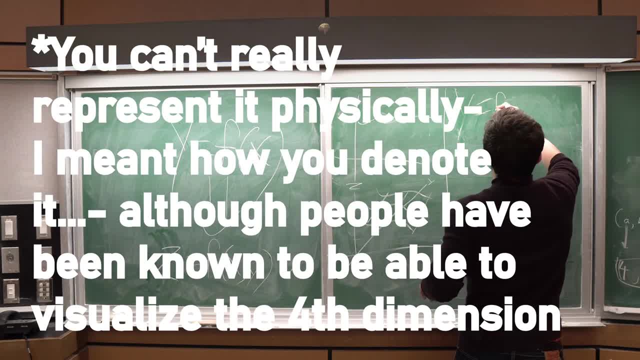 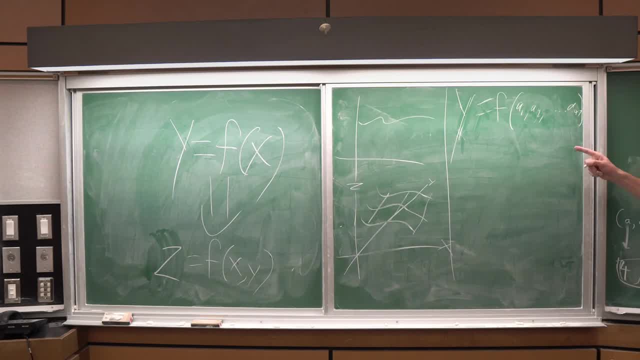 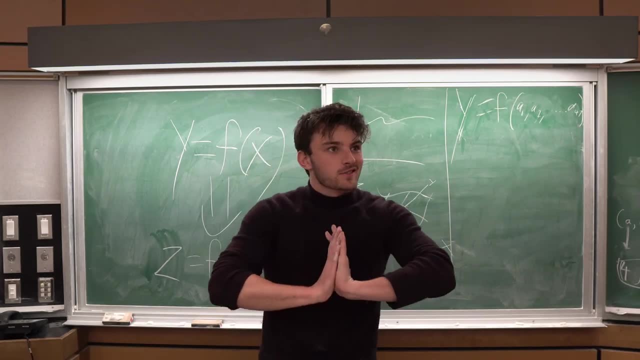 I don't know, like Y equals F of something like that. And they still have idea. They still have one output number. There's one number being output, a bunch of numbers being input. So then some absolute madman, some bad man, descends from the mountain and he goes. guys, I think I want to 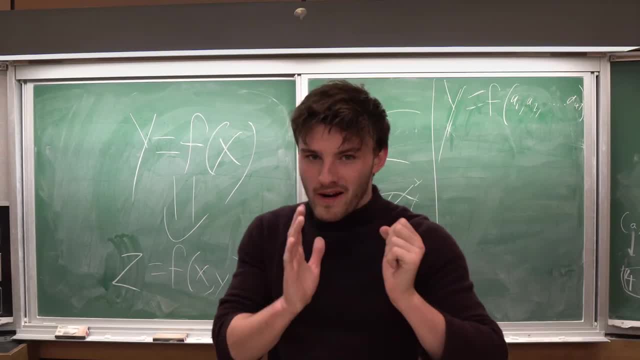 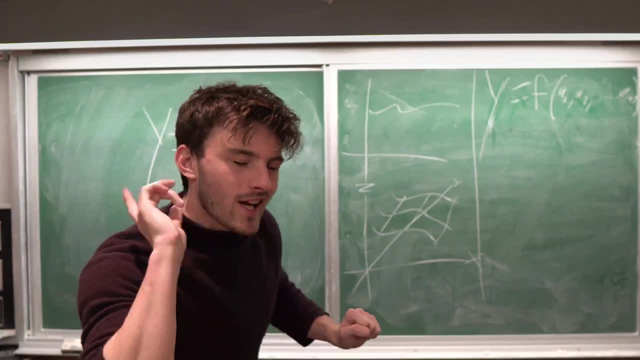 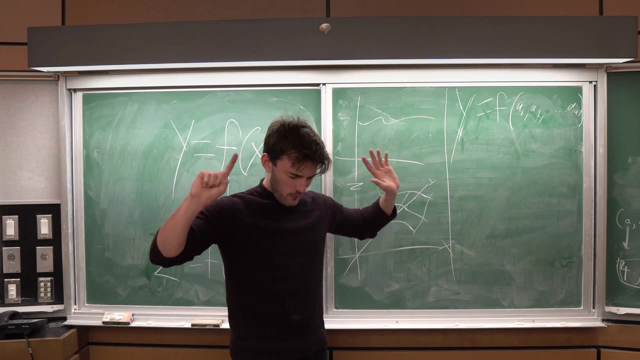 try something out. I want to try something out. up until now You've been in one paradigm, right? You've been thinking: one output, one output number, throw a bunch of stuff in, but one number output. You're not thinking big enough. He's like: all right, why don't we try? Hear me out here. 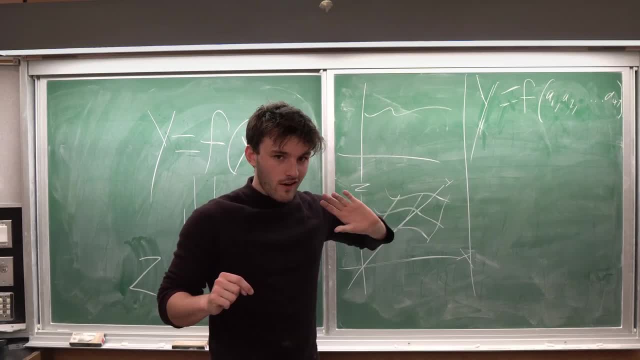 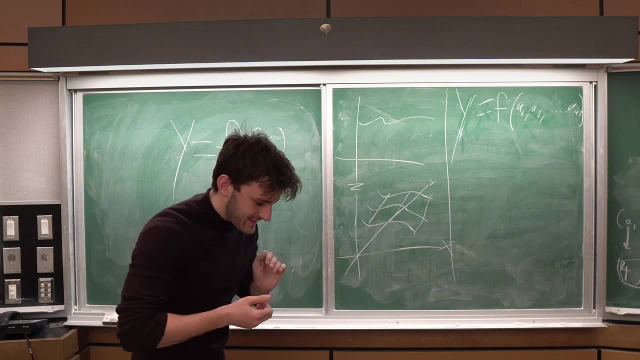 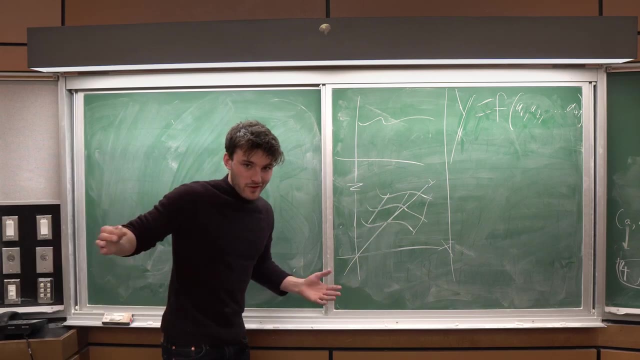 Why don't we try having multiple numbers output as well? And of course, that caused me. Everyone's like: you're a fool, You're a Charleston. Throw this man in the nut house. He clearly needs help, but he's like: hear me out here, Hear me out. So right now he has a room full of people. that's. 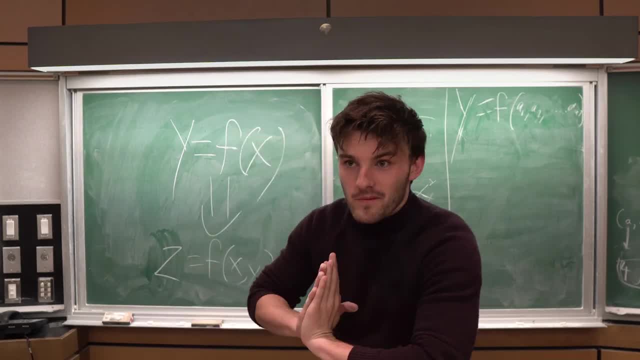 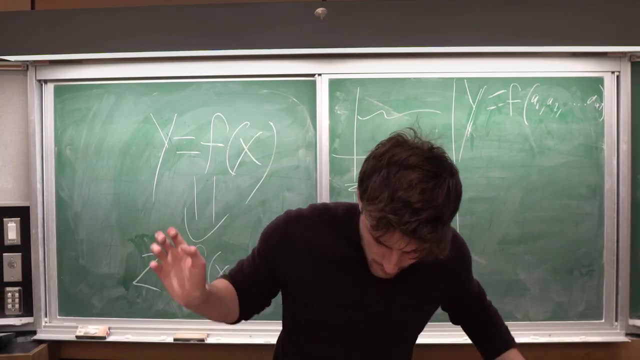 man descends from the mountain and he goes: guys, I think I want to try something out. I want to try something. up until now you've been in one Paradigm, right, you've been thinking: one output, one output number. throw a bunch of stuff in, but one number comes out: one number output. you're not thinking. 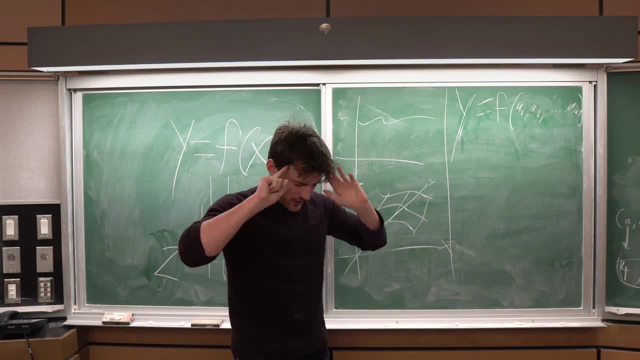 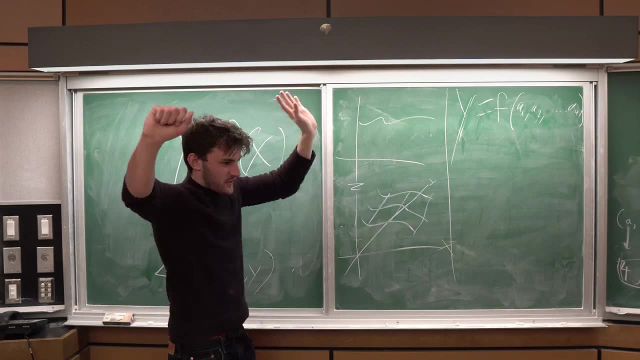 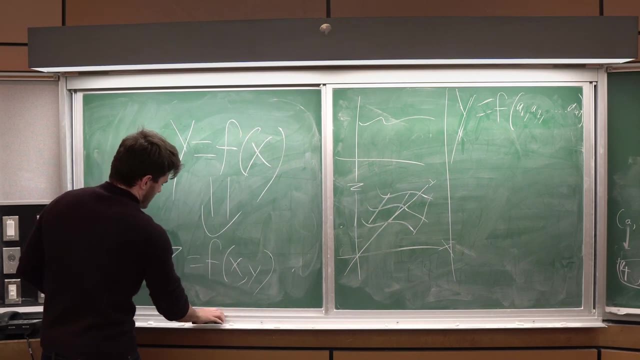 big enough. he's like: all right, why don't we try hear me out here, why don't we try having multiple numbers output as well? and of course, that caused me. everyone's like: you're a fool, you're a charleston. throw this man and then in the nut house. he clearly needs help. but he's like: hear me out here, hear me out. so right now. 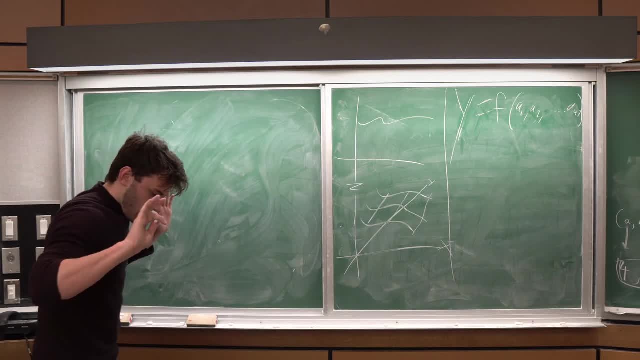 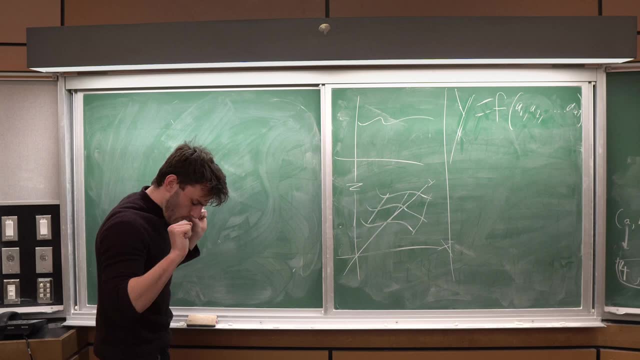 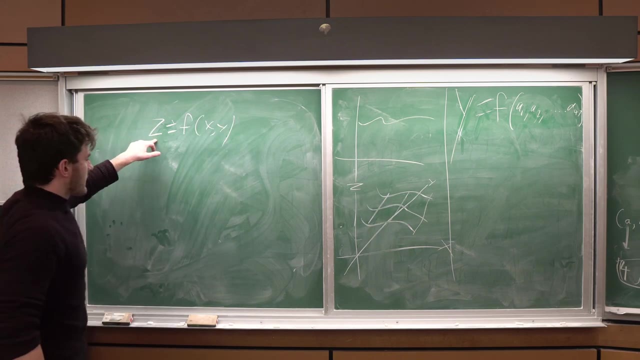 he has a room full of people that's going to decide his fate and he's kind of like: okay, guys, look, right now you have. you know, you accepted that you can have like n-dimensional functions and then one output. right, but what if we for- and let's take the simplest case- what if, instead of having one output, how could we have? 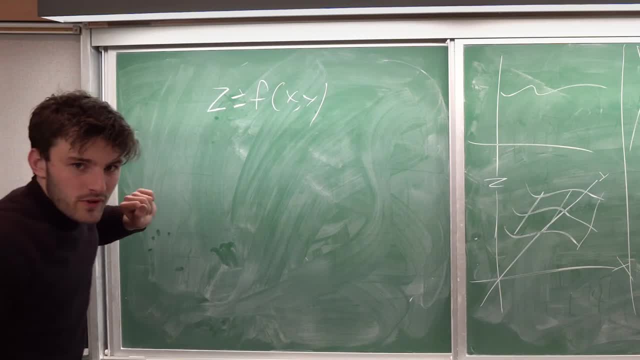 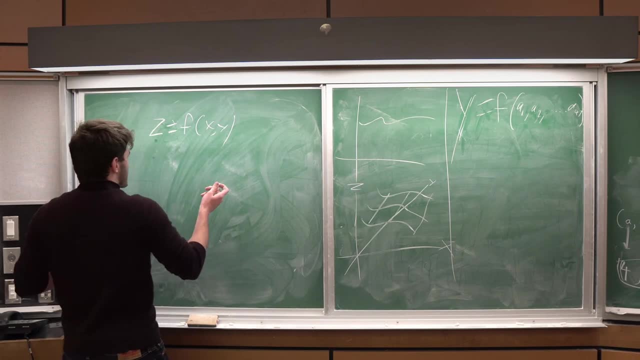 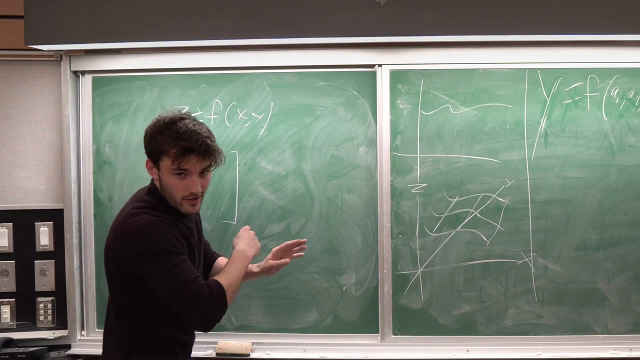 it so that we have two inputs and two outputs. how do we do that? two inputs, two outputs, and so it turns out. the easiest way to do this is to just say: uh, go like this, you want two outputs, right, and so let's say that we're just coming up with this arbitrary notation, we're just trying to. 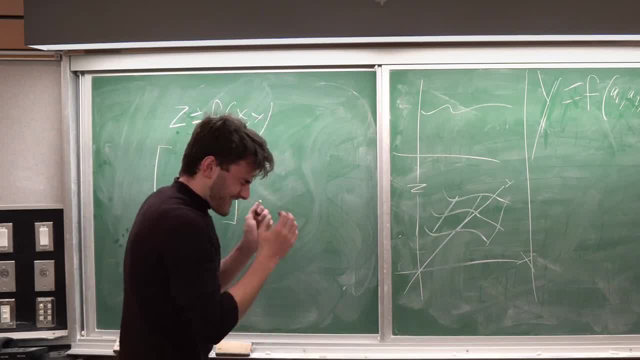 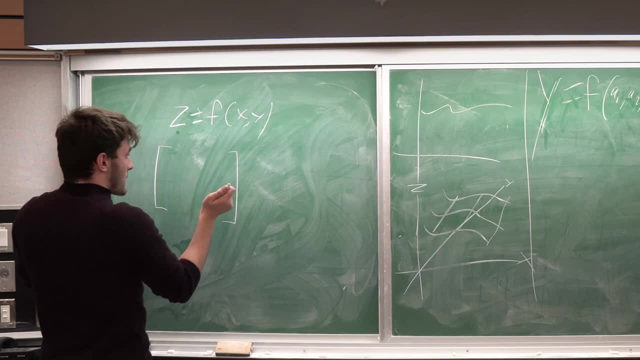 come up with something we haven't operated before. we're just trying to say: okay, how do they represent two-dimensional output? it's a whole whole new thing, right? so he does this. he comes up with this thing and he's like: okay, we're gonna put the first equation up here. I'm gonna say: uh, x, y, let's say g of. 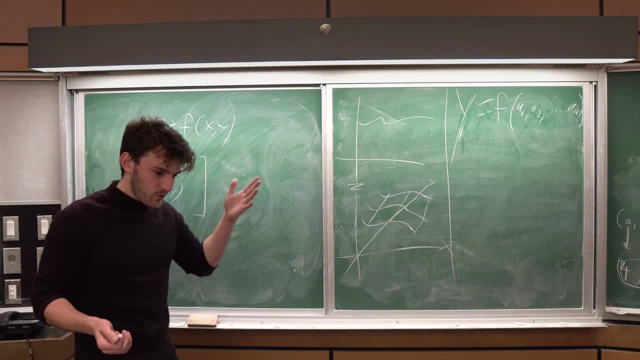 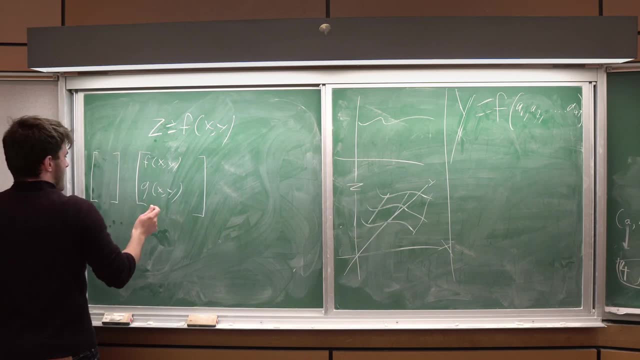 x, y. so we're going to come up with a new notation, because how do you put two numbers as an output to a function? it's all very strange. we're going to have this as uh. we need to call these. I don't know what's the symbol I can use. uh, let's say zw. yeah, we can use zw or wz. 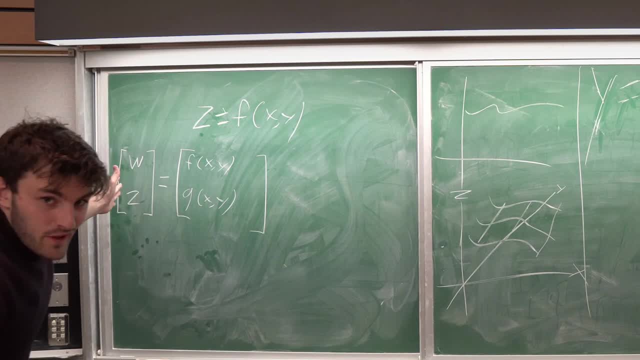 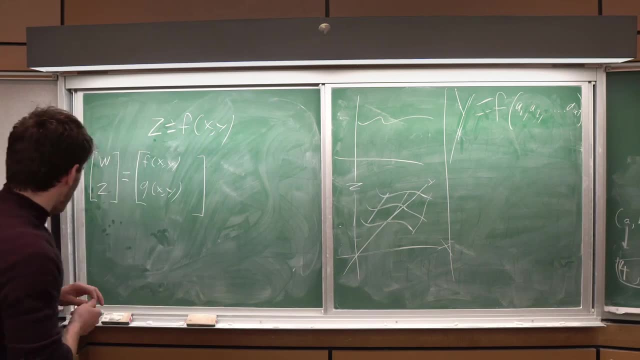 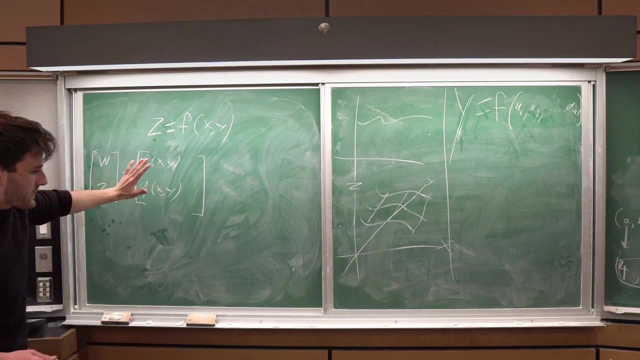 do you feel like you just created a new branch of mathematics because you did bam? multi-dimensional outputs muscle. we have a vector from a vector, so this is is a way of representing a multi-dimensional output and input. so you have two variables, x and y, coming in, and you have two variables coming out. 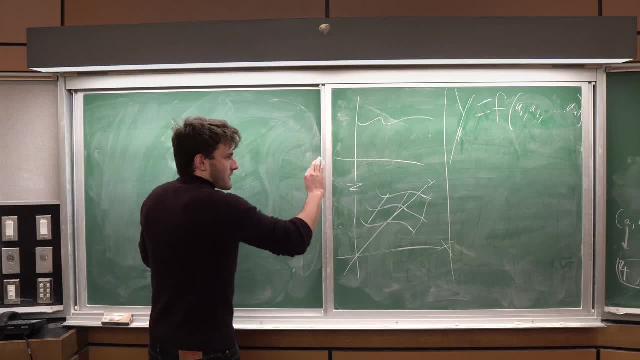 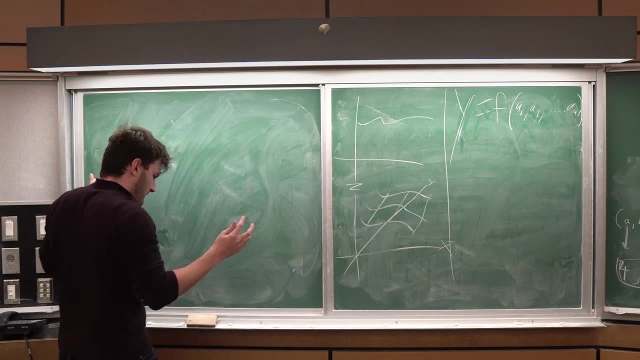 going to decide his fate And he's kind of like: okay guys, look, right now you have, you know, you accepted that you can have like n-dimensional function And then one output, right, But what if we for- and let's take the simplest case- what if instead? 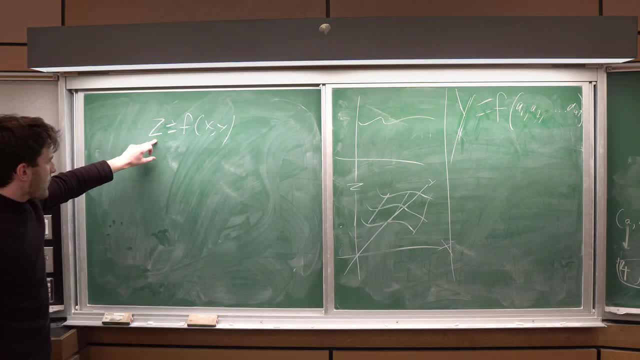 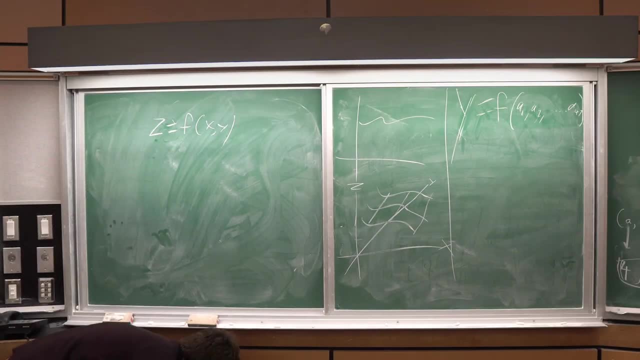 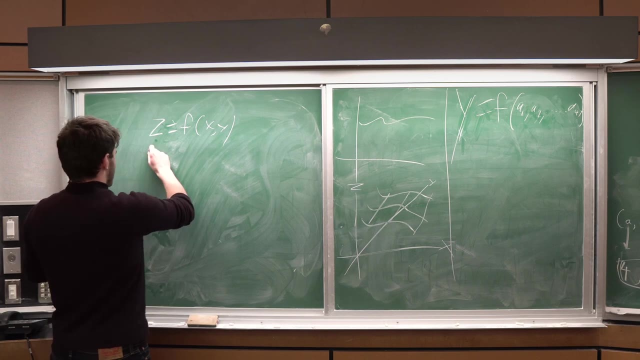 of having one output. how could we have it so that we have two inputs and two inputs? How do we do that? Two inputs, two outputs, And so it turns out. the easiest way to do this is to just say: go like this: You want two outputs, right? And so let's say that we're just coming up with this. 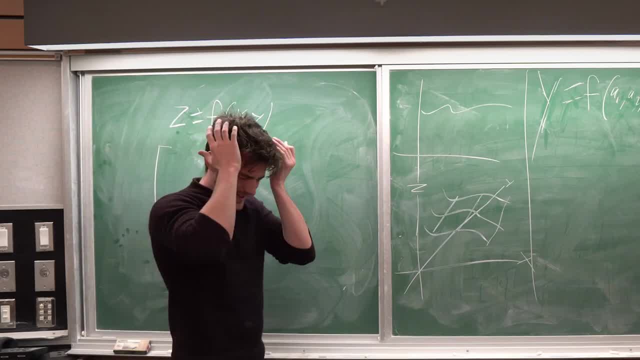 arbitrary notation. We're just trying to do this. We're just trying to do this. We're just trying to come up with something. We haven't operated this before. We're just trying to say, okay, how do we represent this two-dimensional output? It's a whole, whole new thing, right? So he does. 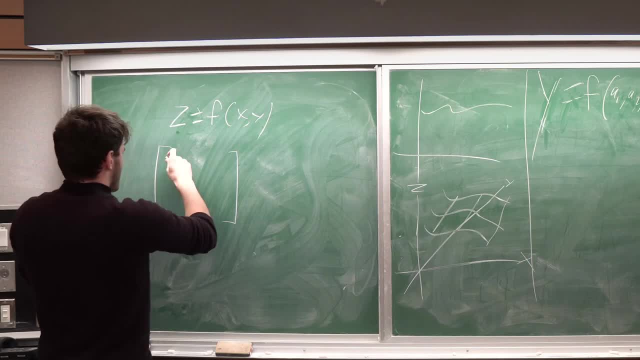 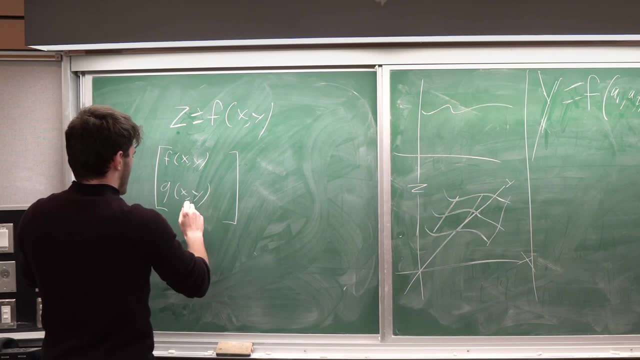 this. He comes up with this thing and he's like: okay, we're going to put the first equation up here. We're going to say x- y, let's say g of x- y. So we're going to come up with a new notation. 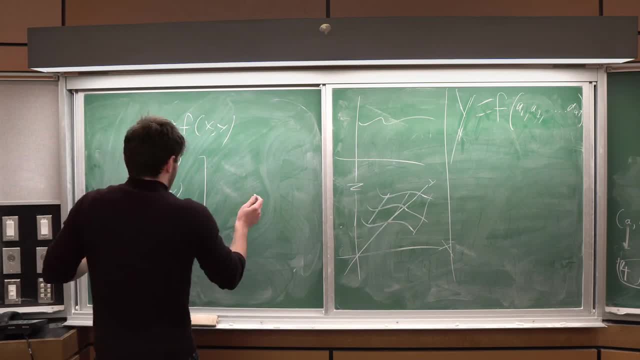 because how do you put two numbers as an output to a function? It's all very strange. We're going to have this as uh. what are you going to call these? I don't know What's a symbol I can use. 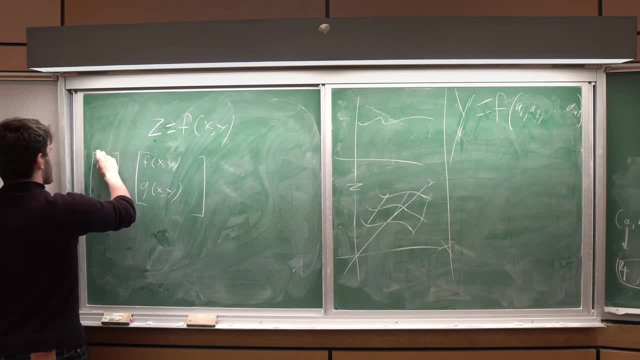 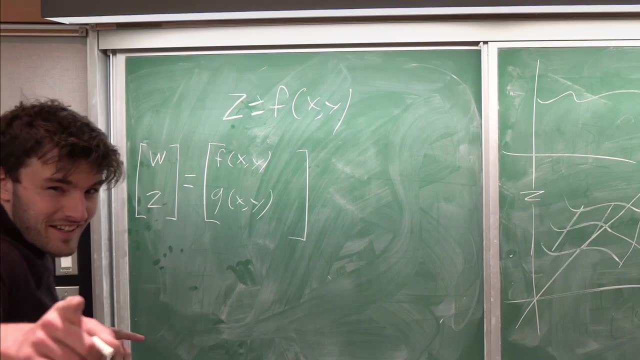 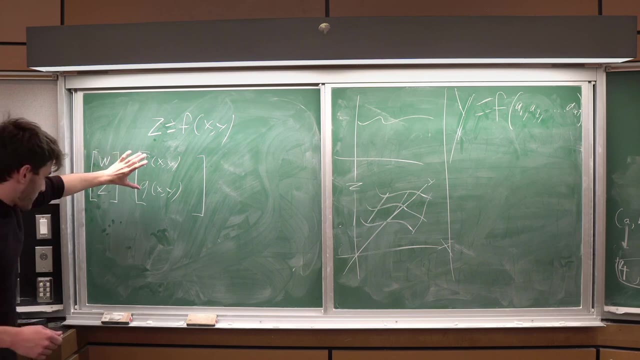 Uh, let's say z w. Yeah, we can use z w or w z. Do you feel like you just created a new branch of mathematics? Cause you did Bam. Multi-dimensional outputs. So we have a vector from a vector. So this is a is a way of representing a multi-dimensional output, and 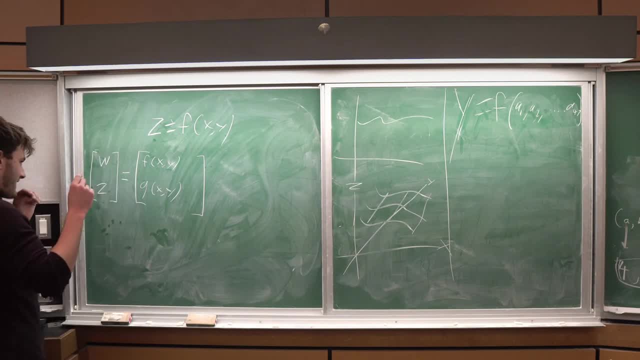 input. So you have two variables, x and y- coming in, and you have two variables coming out. And let's, let's- there's another way of representing this- Let's go, uh, cause this is. I mean, this is kind of 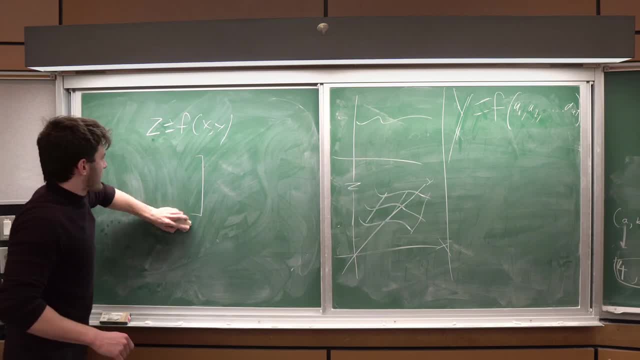 here. We've just invented this on the spot, Uh, so over time, you know you have, we want to put it in normal function notation, Um, and so instead of that, we're going to have, uh, let's say just: 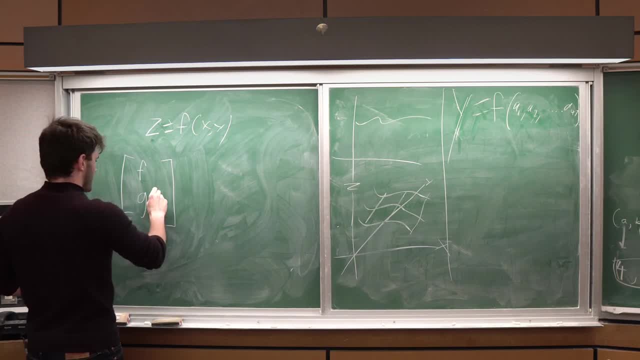 put f of f here and g of here. These are functions We're going to have. uh, maybe put them like that. I don't know. Kind of poor notation, but we're working with notation here, So it's all good. 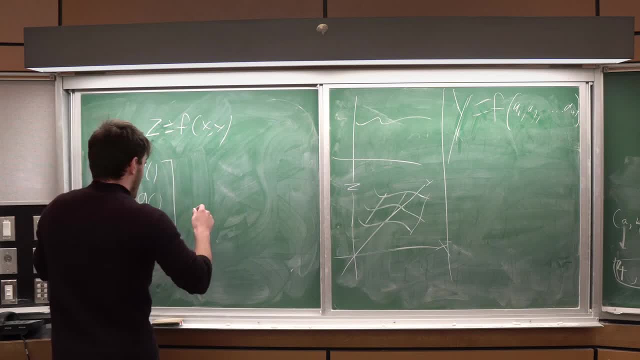 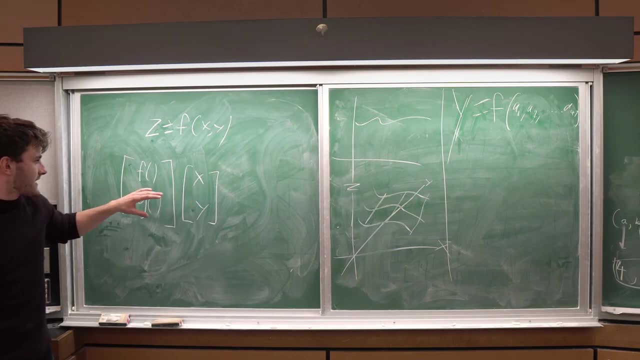 We're inventing notation Um, and then, because we have two inputs going in, we're going to put them like this, And so all this means is like go like this: Right, So f of something and then find out whatever that is, and g of this and find out whatever that. 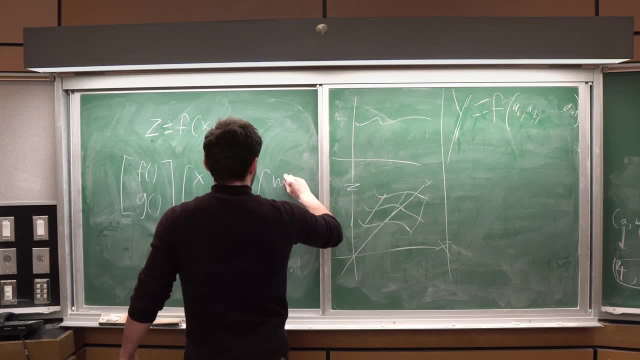 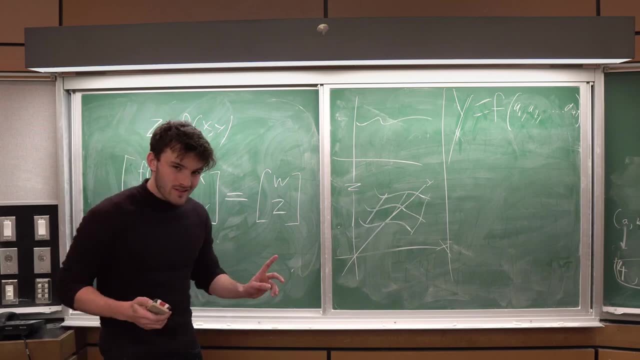 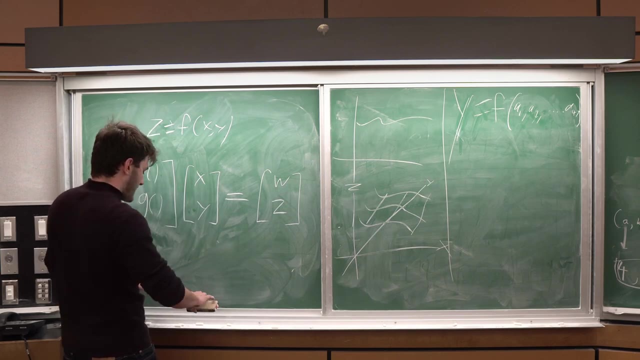 is Um, and so we're going to say equals. So that's how you represent multi-dimensional outputs for multi-dimensional inputs, And then hopefully you're noticing some similarity between this and matrices. We're almost there. So matrices are just this And and and. with this, you can. you can. 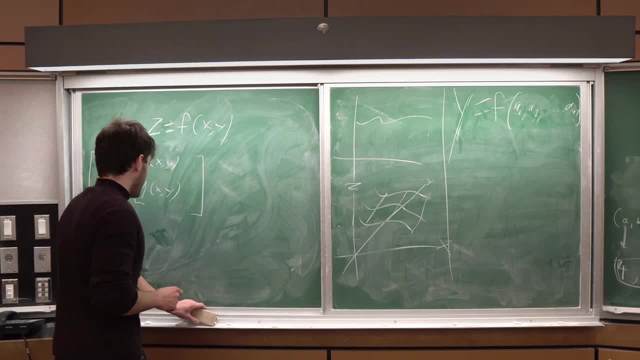 and let's, let's- there's another way of representing this. let's go, uh, because this is- I mean, this is I don't know- kind of here, we've just invented this, we've just invented this, we've just invented this on the spot. uh. so over time, you know you have to, we want to put it in the normal function notation. 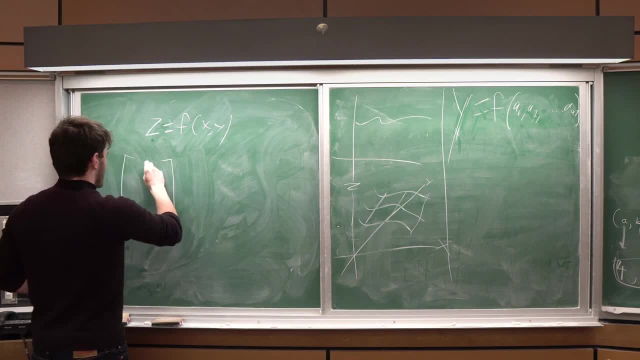 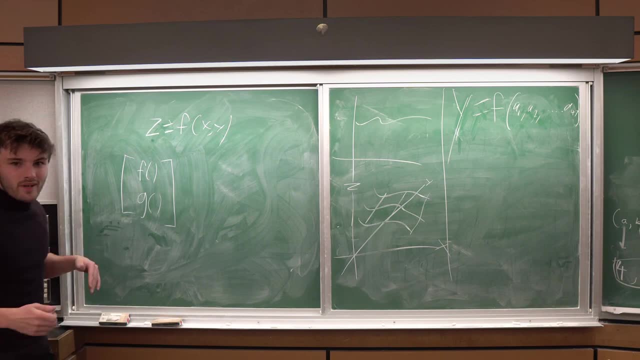 um, and so instead of that, we're going to have, uh, let's say, just put f of f here and g of u. these are functions we're going to have- uh, maybe put them like that, I don't know- kind of poor notation, but we're working with notation here, so it's all good. we're inventing notation um, and then, because 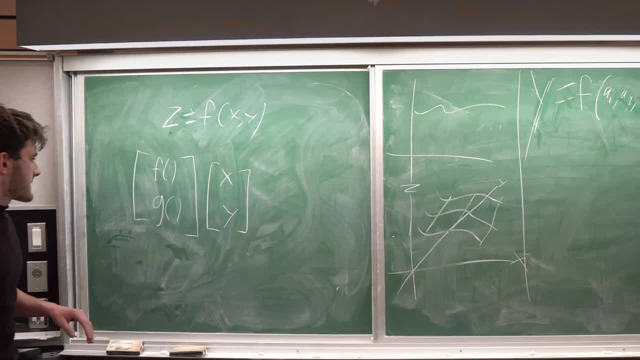 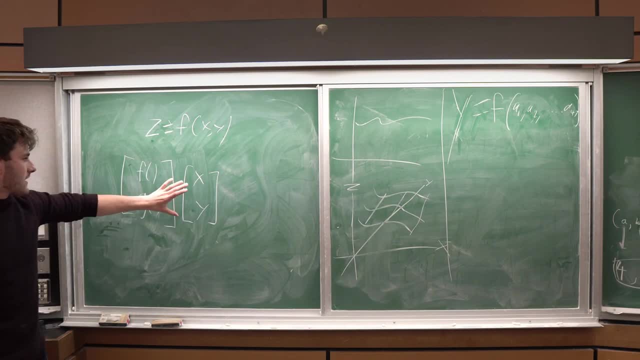 we have two inputs going in. we're gonna put them like this, and so all this means is like go like this, right, so f of something and then find out whatever that is, and g of something and then find out this and find it whatever that is, and so we're going to say equals. 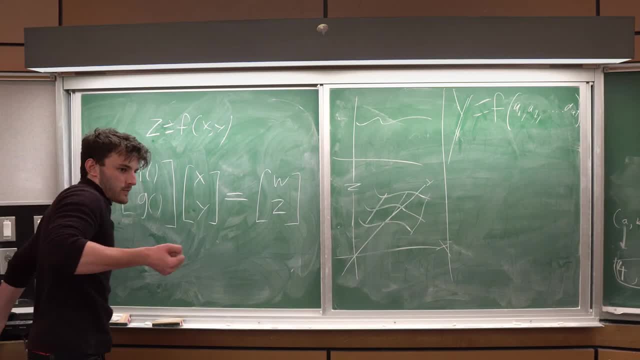 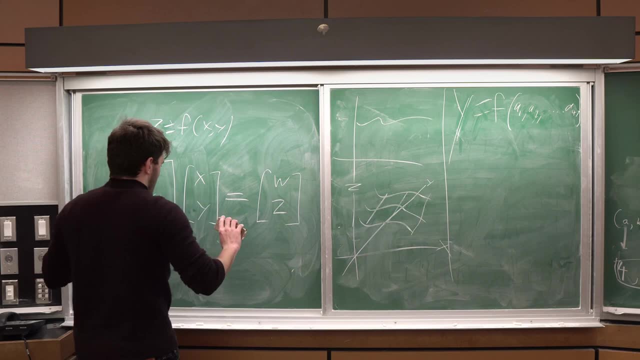 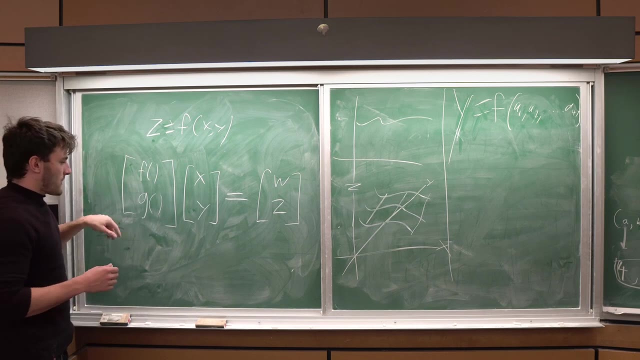 so that's how you represent multi-dimensional outputs for multi-dimensional inputs, and then hopefully you're noticing some similarity between this and matrices. we're almost there. so matrices are just this, and and with this you can, you can go, I don't know. you have like 20 inputs and 20 outputs, or like two inputs and 14 outputs. like you can, you can make. 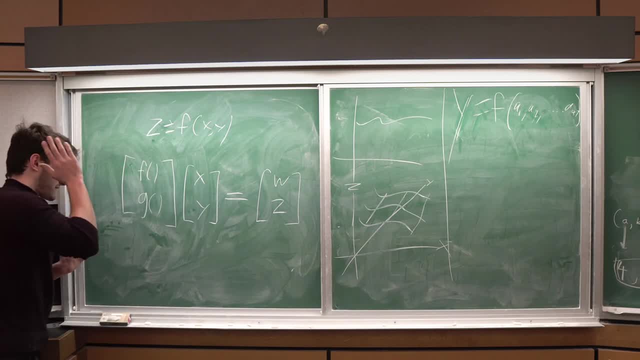 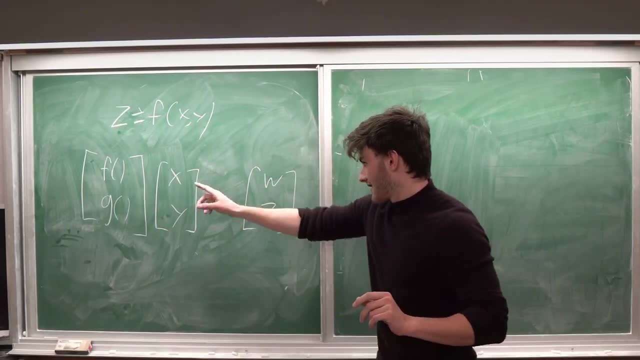 these crazy, stupid, but at the end of the day it's a function. we're operating with functions, function, It's a function, And so all a matrix is also. there's a way of representing this thing. Watch 3Blue1Brown's linear algebra series. 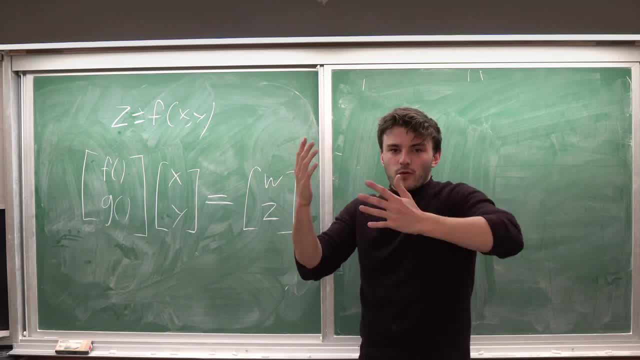 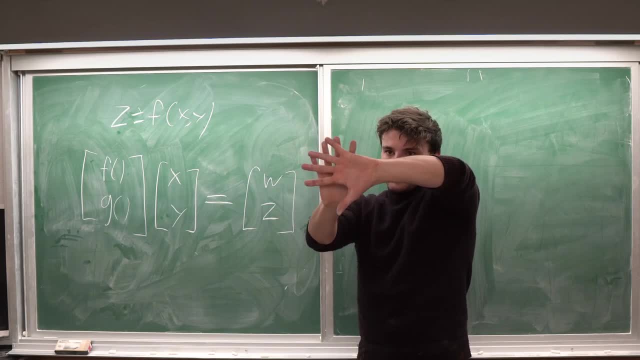 It's like you take a so say it's a two-dimensional, two-dimensional, It's a four-dimensional thing what you're operating with. but you can kind of take the original graph, superimpose a new graph on top of it and then wherever the lines go. 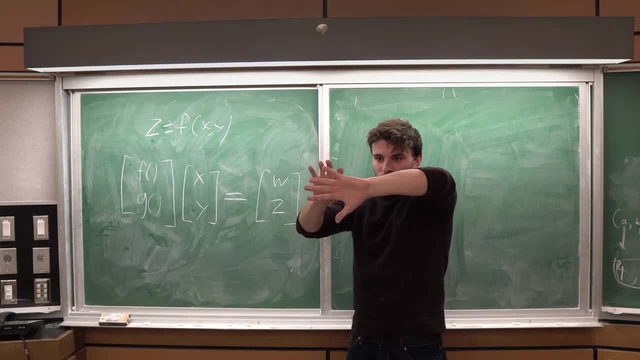 that becomes like the new point. So it's like the function takes the point one one and moves it to like 13, 14.. It'll like: move it over there. But watch 3Blue1Brown, you'll see what I'm talking about. 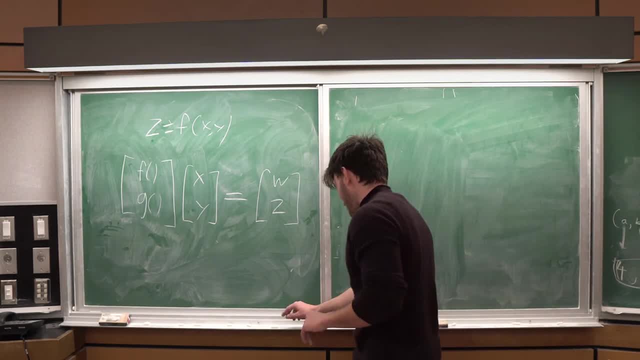 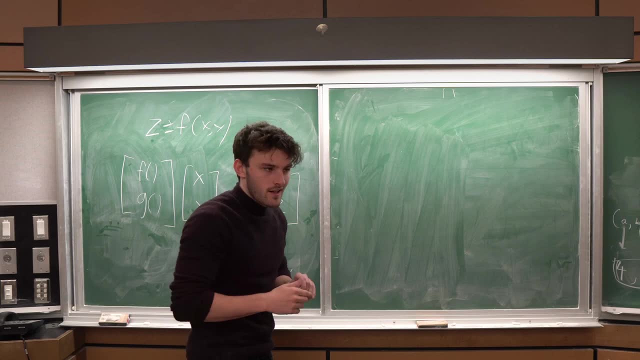 I don't have the technology at this point to do my own. Okay, So then the only next step we're going to do is limit this to linear equations. So linear equation, a linear equation is any equation that just multiplies it by some number. 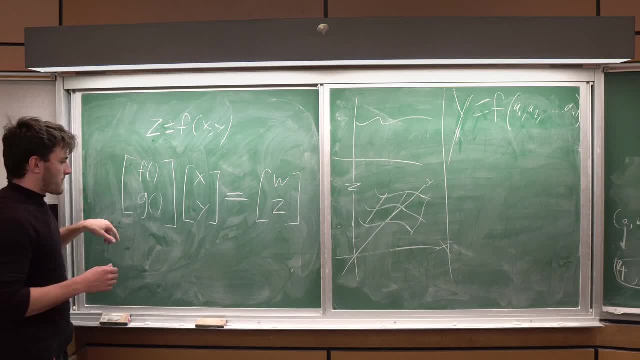 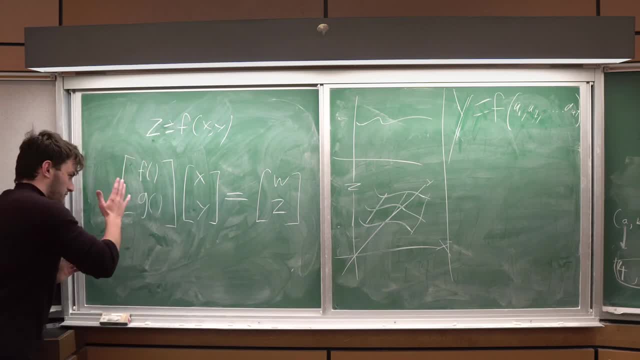 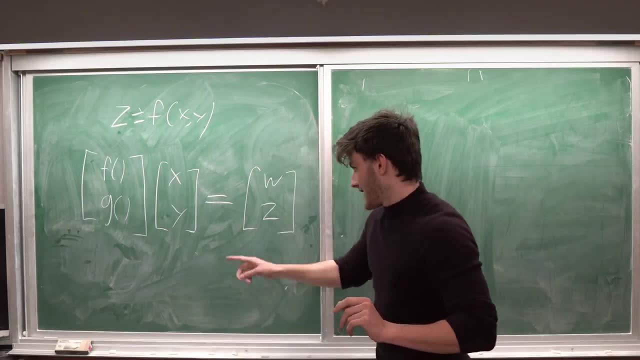 get crazy stupid, but at the end of the day it's a function. we're operating with functions, function, think functions function, And so all a matrix is. oh, also, there's a way of representing this thing. Um, watch three blue one Brown's uh linear algebra series. It's like you take a. 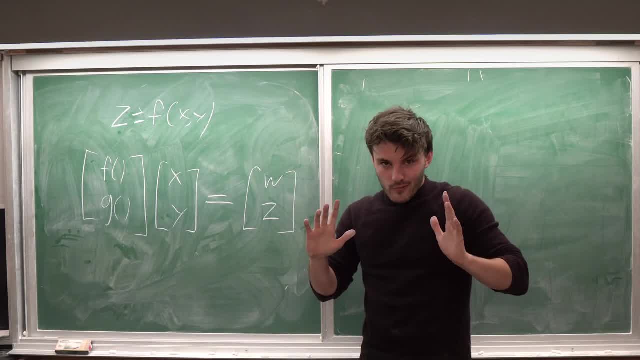 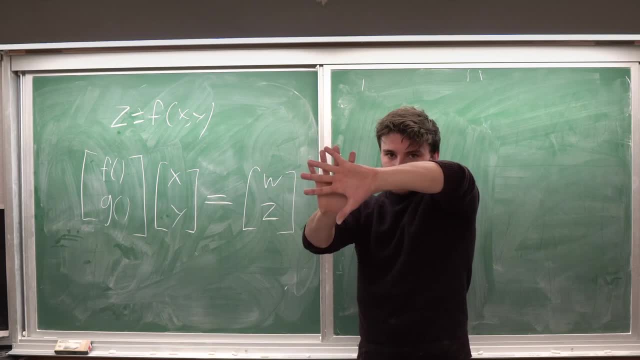 so it's a. it's a two dimensional, two dimensional, It's a four dimensional thing what you're operating with. but you can kind of take a, take the original graph, superimpose a new graph on top of it And then wherever the lines go, that. 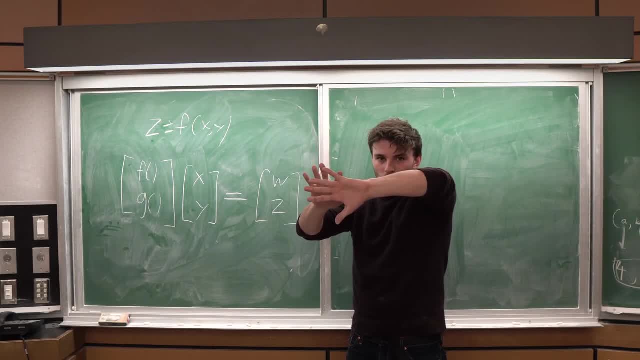 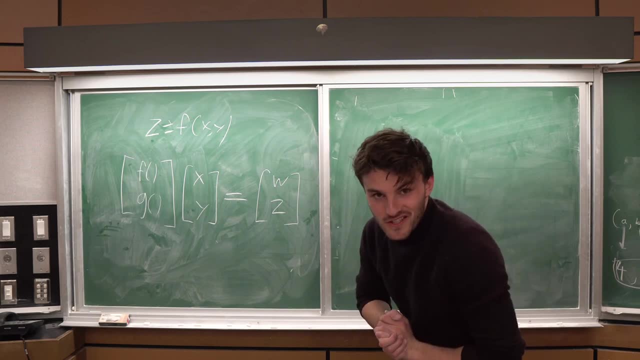 Like the new point. so it's like the function takes the point one, one and moves it to like thirteen, fourteen. It'll like: move it over there. But what? three blue, one brown? just you I'm talking about. I don't have the technology at this point to do my own. 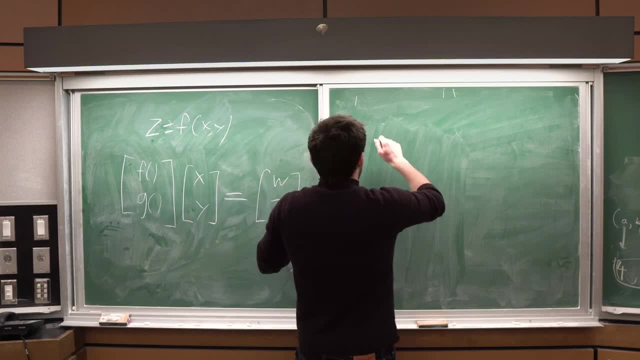 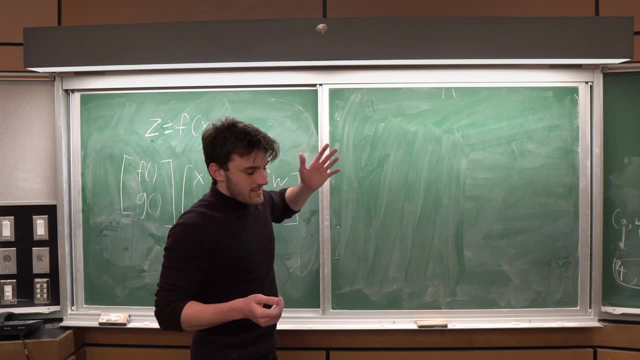 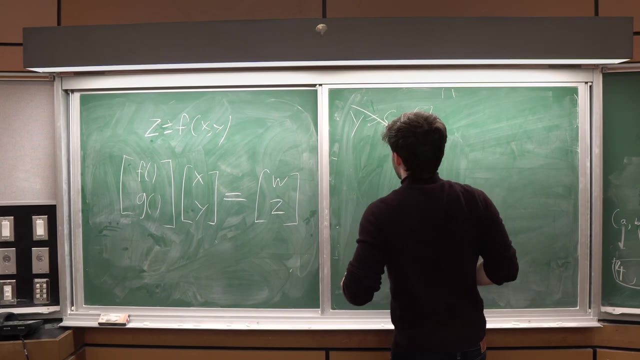 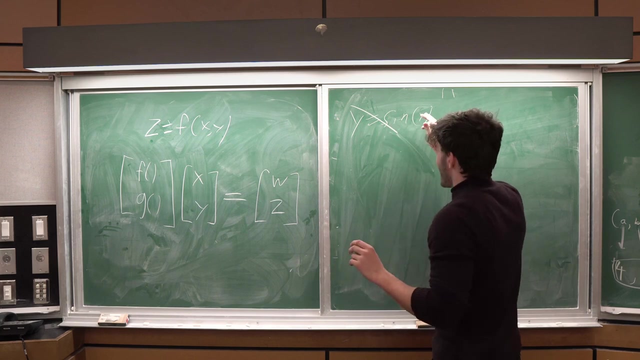 Okay. so then the only next step we're gonna do is limit this to linear equation. So linear equation, a linear equation is any equation that just multiplies it by some number. So y equals sine of X, Not linear, not linear, not multiplying by some Coefficient. right now It's just not just a nice easy: y equals blank of X, It's y equals sine of X. It gets all curvy. 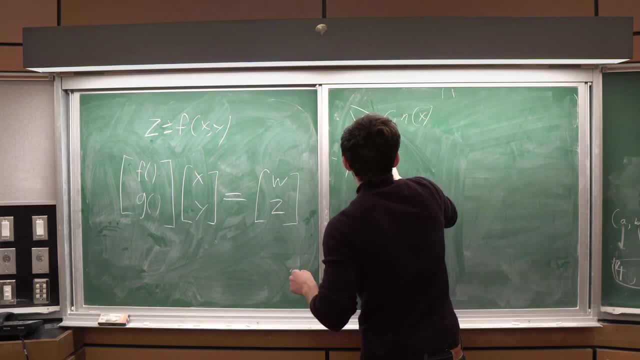 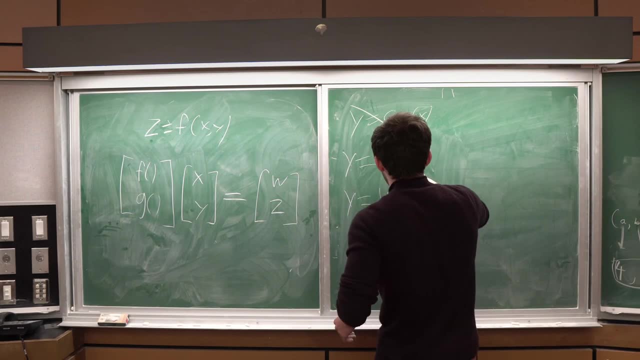 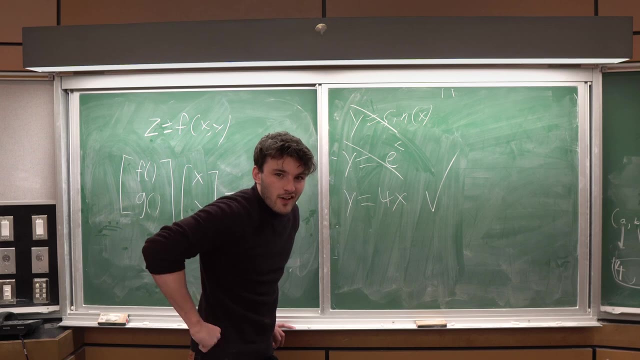 wrong, incorrect, not linear. y equals e to the X, not linear. unfortunately, y equals 4x. That's linear. linear because It's a long, it's a line and also the coefficients aren't allowed. I Had a big problem of this, like: what? what about? y equals 4x? 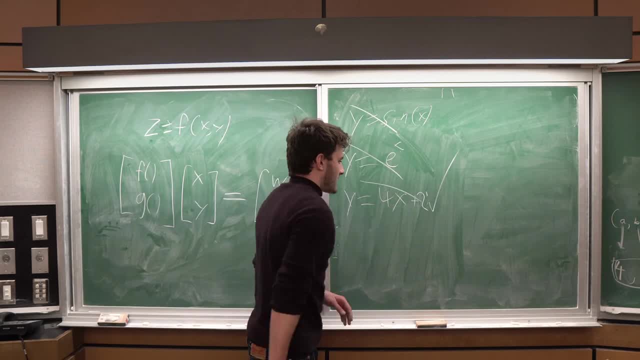 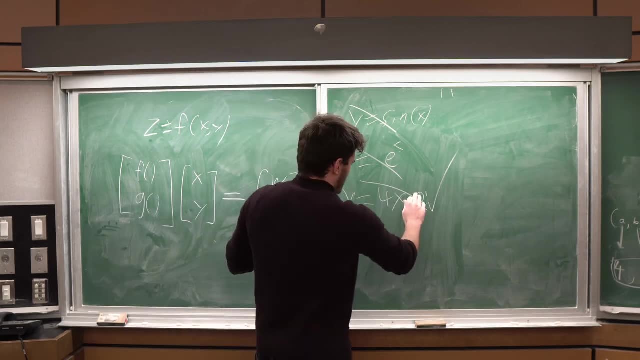 Plus 2. why? what about that? and that actually turns out not to be fitting. our thing is the whole. I don't bit of this. Why that's the case. It's very complicated, but just this is what you don't know. not allowed, allowed to have like plus twos on it some. 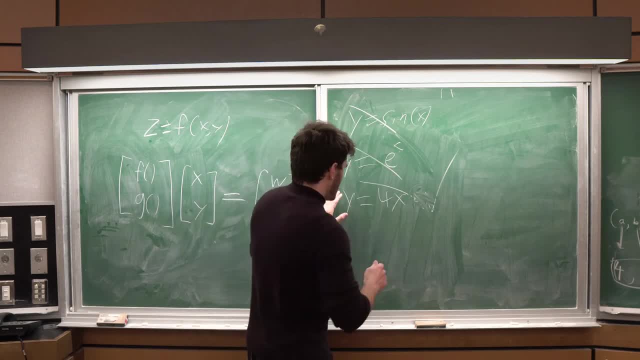 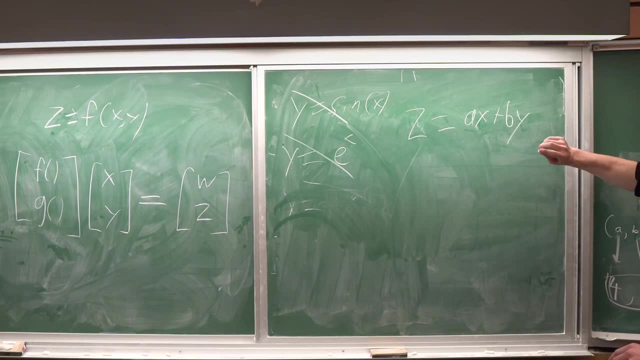 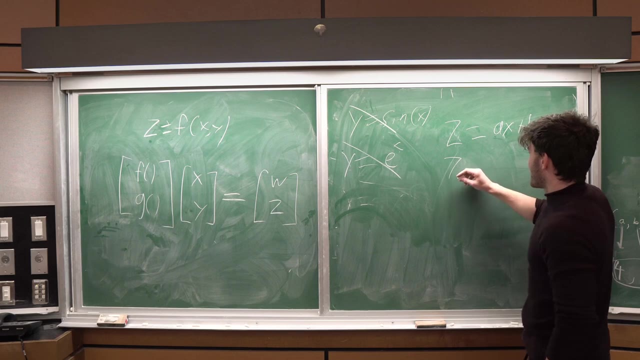 number multiplied by the variable. that's a linear function. a multidimensional linear function is equals, So it's just coefficients multiplied by the variable. So this is a, this is yep, That's good if they and B are. are just normal numbers Or not normal, just numbers. They don't need to be normal numbers. 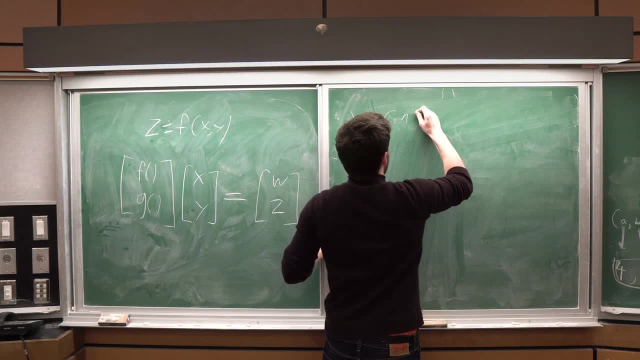 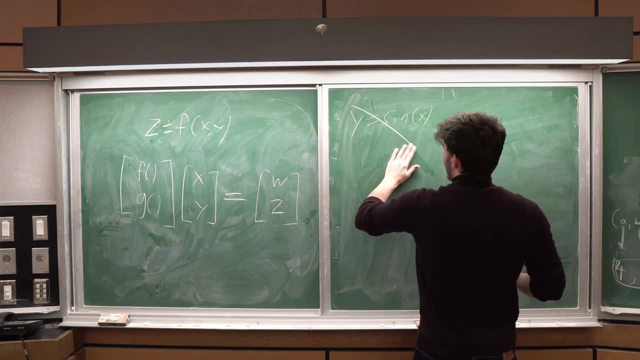 So y equals sine of x, not linear, not linear, Not multiple. It's multiplying by some coefficient, right? It's not just a nice easy y equals blank of x. It's y equals sine of x. It gets all curvy. 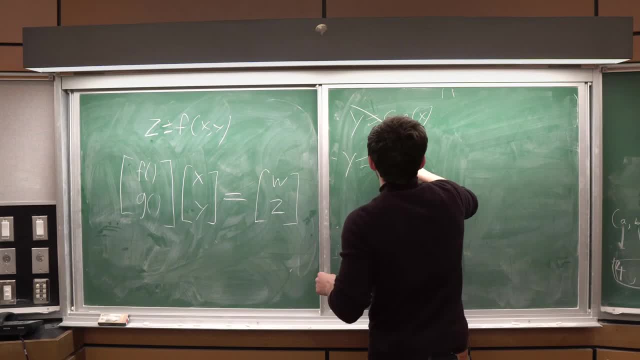 Wrong, Incorrect, Not linear. Y equals e to the x, Not linear, unfortunately. Y equals 4x. Hold on, That's linear, Linear, Because It's a line. It's a line And also coefficients aren't allowed. 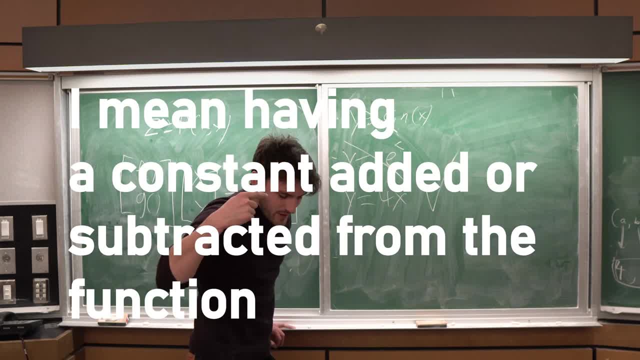 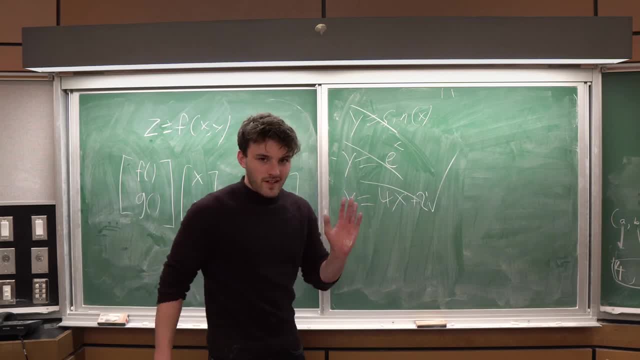 I had a big problem with this, Like: what about y equals sine of x Linear? Because It's a line, Y equals 4x plus 2. What about that? And that actually turns out not to be fitting our thing. 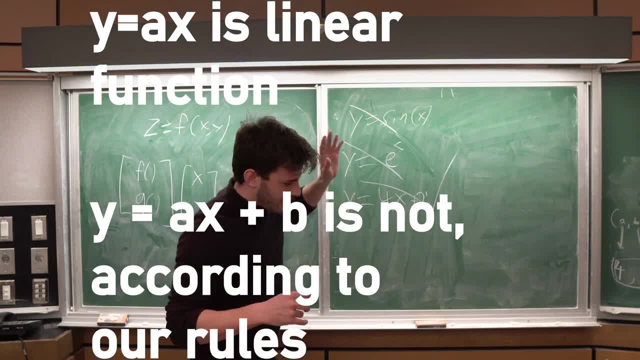 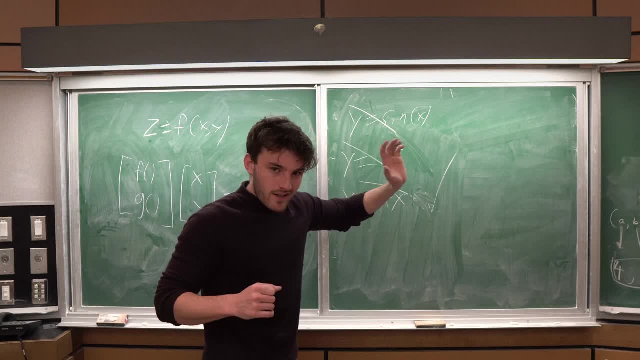 It's a whole. I dove into this. Why that's the case. It's very complicated, But just, You're not allowed to have like plus 2s on it, Some number multiplied by the variable. that's a linear function. 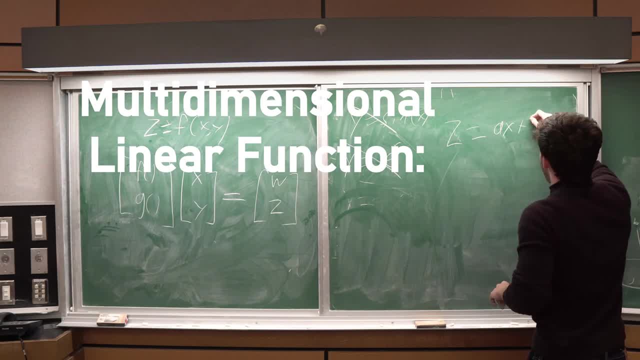 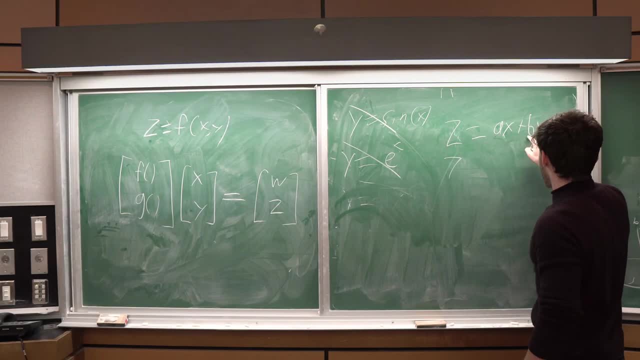 Multidimensional linear function is equals, so it's just coefficients multiplied by the variables. So this is a, this is yep, that's good. The a and b are just normal numbers Or not normal, just numbers. They don't need to be normal numbers. 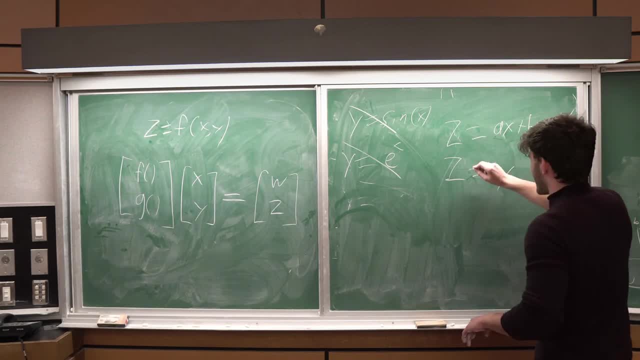 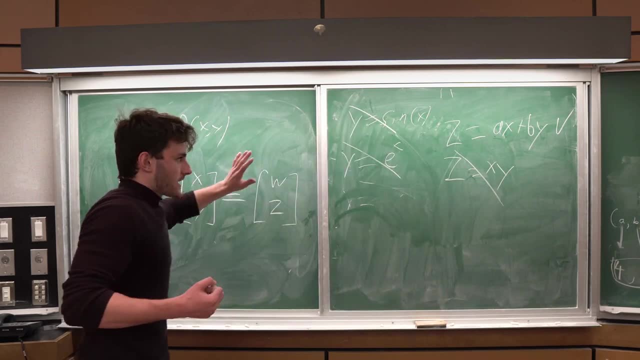 Just real numbers. sorry, But this, This is no good. That's not linear, That's not linear. Unfortunately, Not linear Does not make a cut. Okay, So you have linear numbers and you have multidimensional functions, Or sorry? 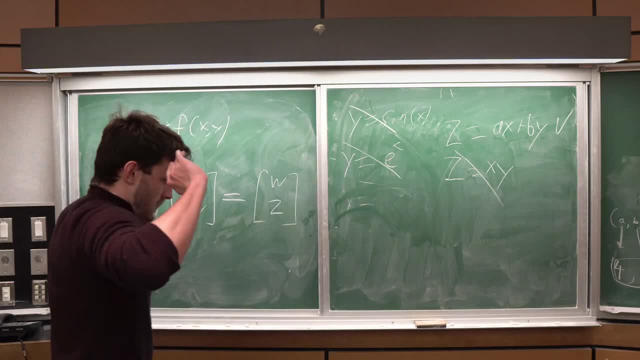 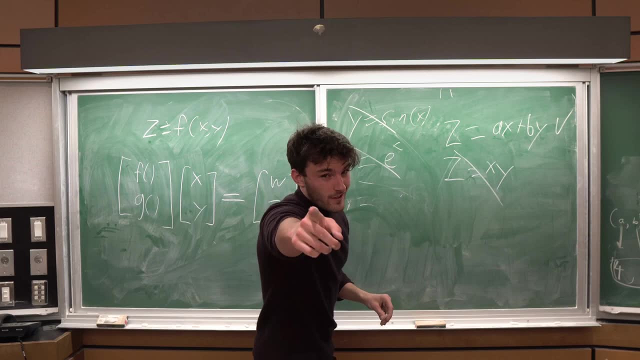 You have linear functions and multidimensional functions. Linear functions, Multidimensional functions, Peanut butter and chocolate. time You ready, Bring them together. What do we got? What do we got? What do we got? What we got is matrices, baby. 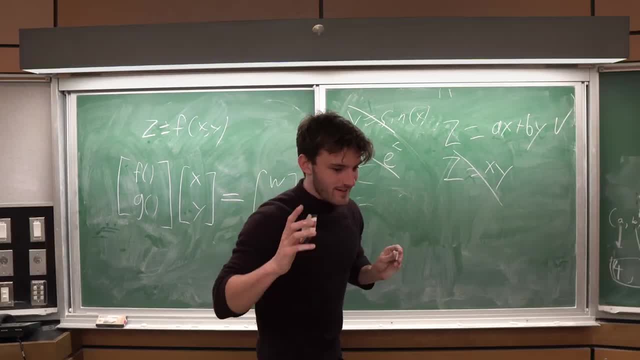 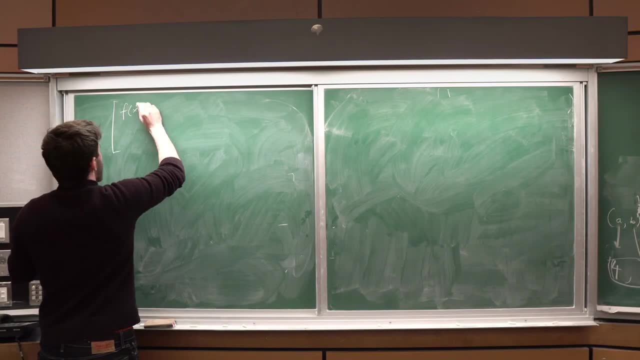 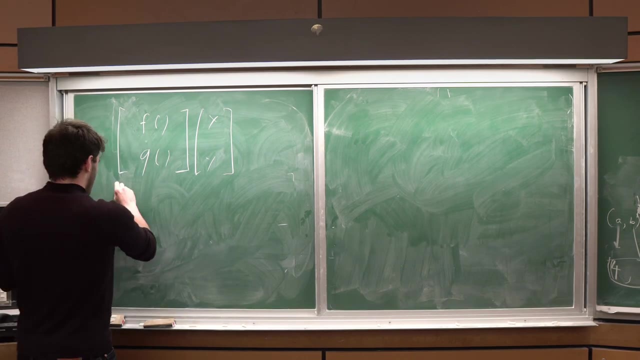 When you see a matrix, think function. Matrices are functions. They take in vectors and they spit out vectors. Vector comes in, Spits out a vector. So matrix is just this or some larger version of this. So maybe it's like it can be three long. 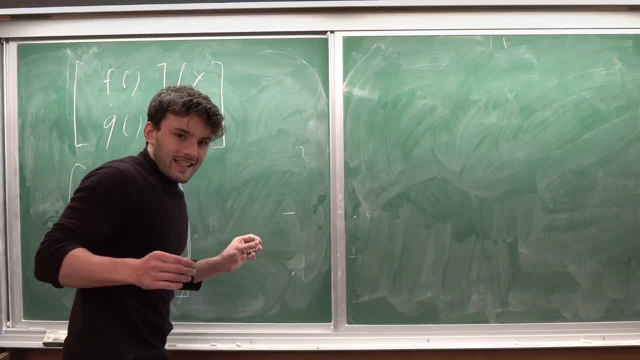 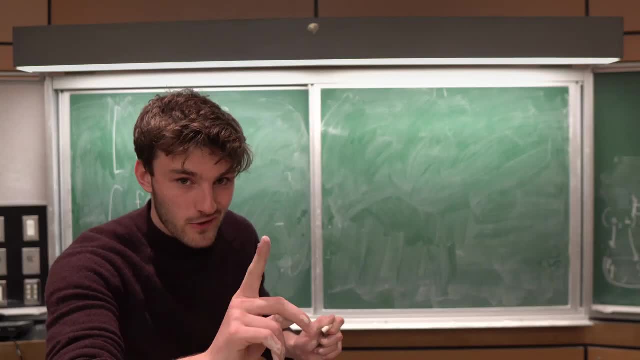 It. it could be arbitrarily long and taken arbitrarily sideways Vectors, but the other day it's just a way of doing multi-dimensional linear outputs. So you take it takes a vector in, spits a vector out and it does so linearly. that's the trick. 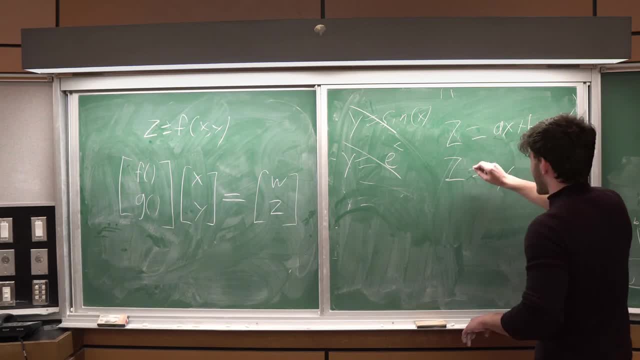 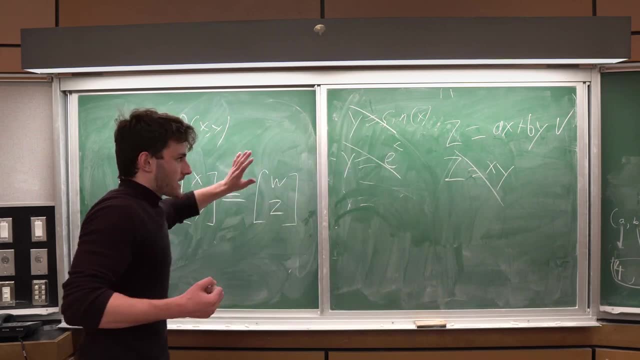 Just real numbers. Sorry, but this, This is no good. That's not linear, We're not running, There's no linear. Unfortunately not linear does not make the cut. Okay, so you have linear numbers and you have multidimensional functions- right? 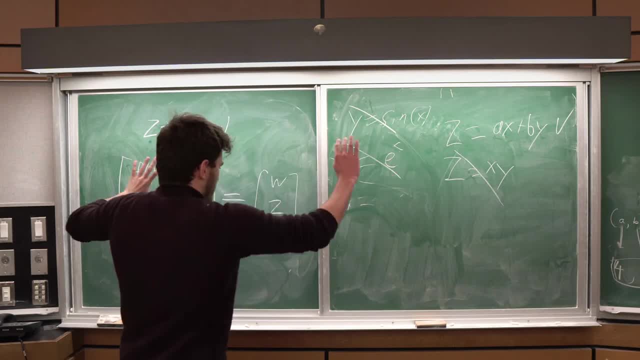 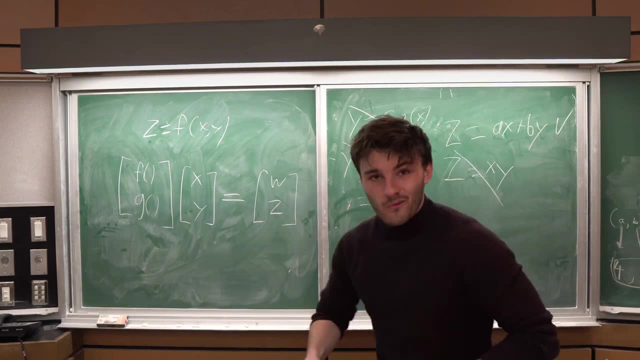 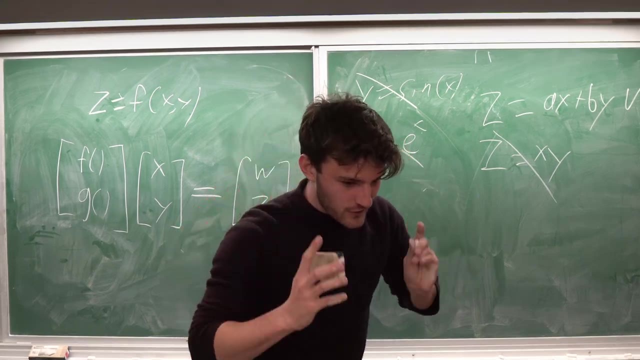 Sorry, you have linear functions and multidimensional functions. linear functions, multidimensional functions, peanut butter and chocolate. time You ready, Bring them together. what we got? What do we got? What we got is matrices, baby. When you see a matrix thick function, matrices are functions. they take in vectors, They spit out vectors. vector comes in. 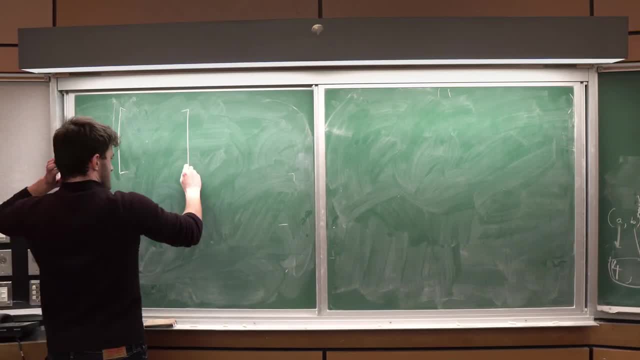 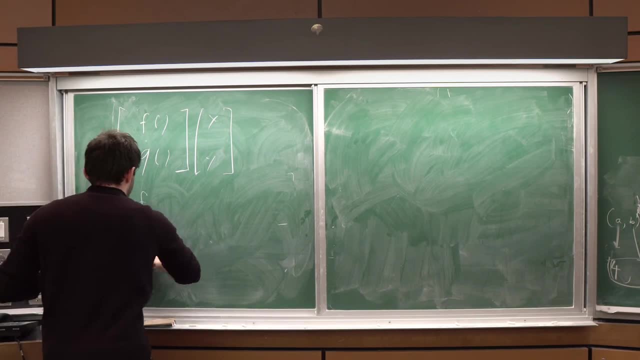 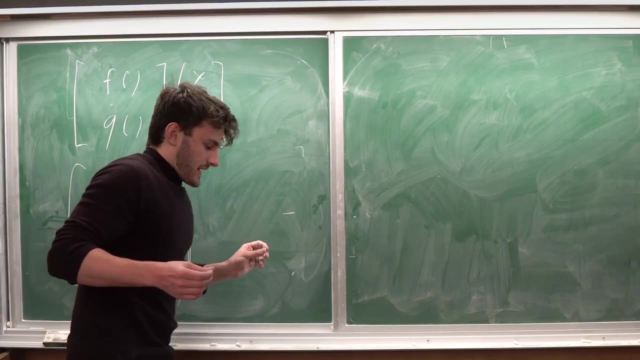 spits out a vector. So matrix is just this or some larger version of this, so maybe it's like It can be three long. it could be arbitrarily long and taking an arbitrary size vector, But the other day it's just a way of doing multidimensional linear outputs. 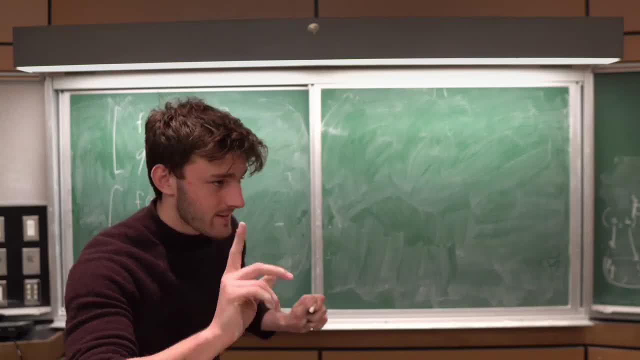 So you take it takes a vector in, spits a vector out and it does so linearly. That's the trick. It's like it's a, it's a way of doing multidimensional functions, And the only restriction on that is it's linear, the linear way of doing it. 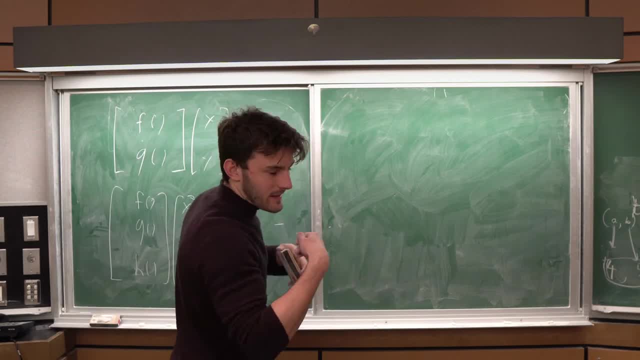 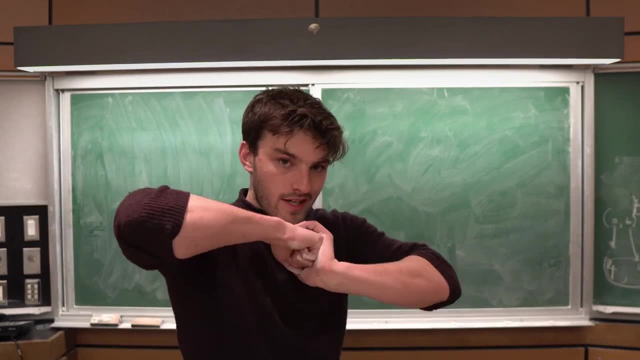 So it does the- I erased it, but it does it multiply to be variable by some number, Because it just does the linear thing. there's an easier way of representing it: You can just put the coefficients in the actual function notation, And so we do that by like, okay. 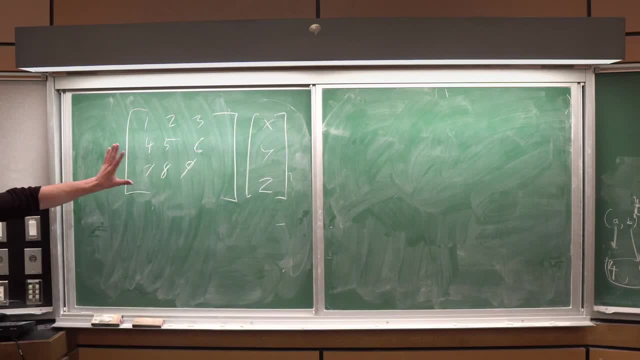 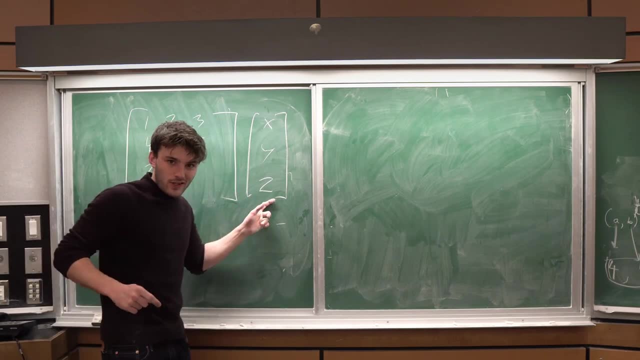 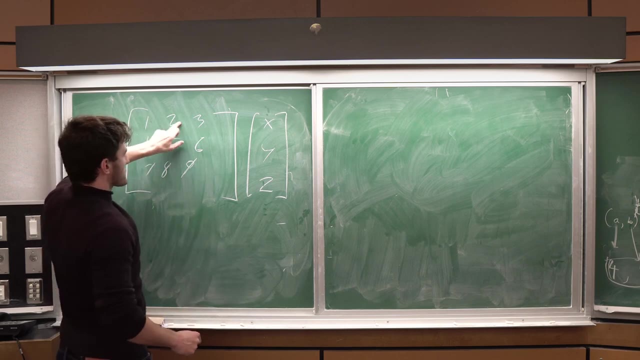 So what this says, What this says, that took me forever to understand. this is just a function. It's just a function and it takes in these, this thing. This is the argument. This is the argument and this is the function. this says: take this right: XYZ. take X multiply by 1. take Y multiply by 2. 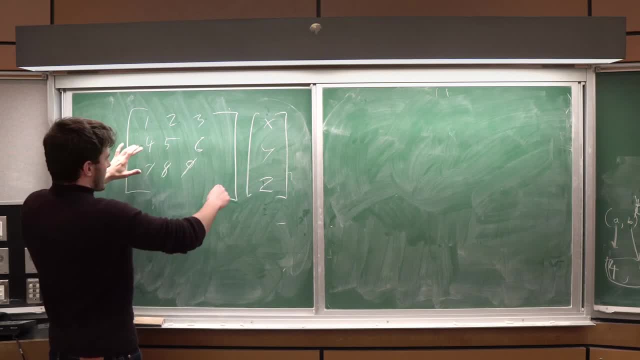 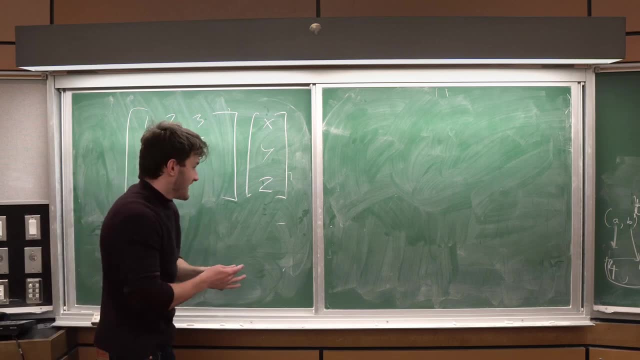 Take Z multiply by 3. same thing for this row. take 4 multiply by Y. take 5 multiply by. Oh shit, no, take 4 multiply by X, Sorry. take 5 multiply by Y. take 6 multiply by Z. And we just invented this. we invented this notation, this way of multiplying it. 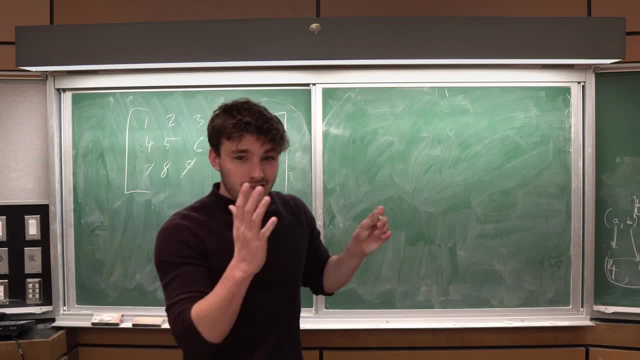 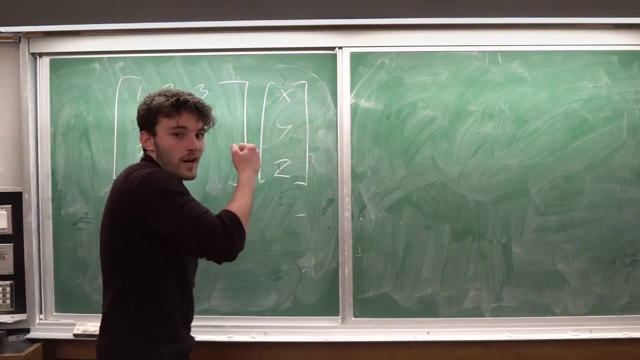 It's just a way of doing it. I mean, come up with your own way of trying to take a vector as an input and have a vector as an output, Just to see how you can do it. There's a ton of ways to notify it. This is just one we've come up with, but it's just an arbitrary way of writing it down. 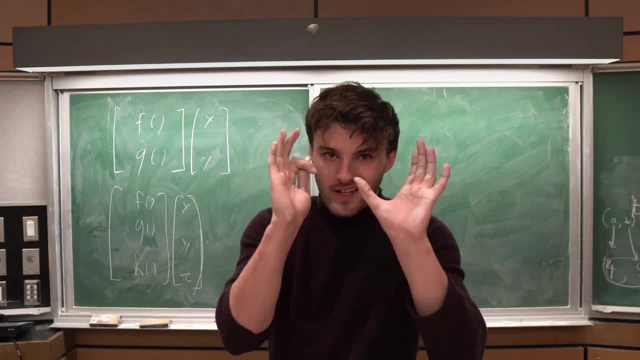 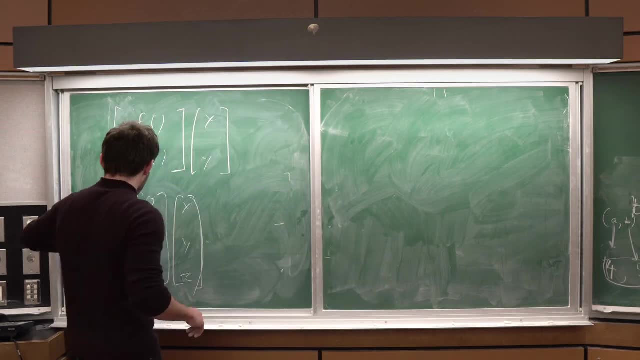 It's like it's a. it's a way of doing multi-dimensional functions And the only restriction on that is it's linear, the linear way of doing it. So it does the. I erased it, but it does. it multiplies every variable by some number. Because it just does the linear thing. there's an easier way of representing it. 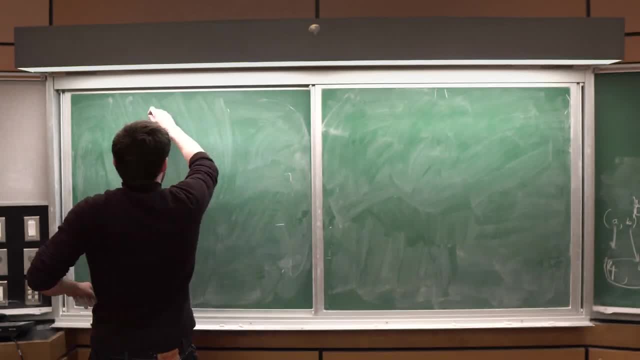 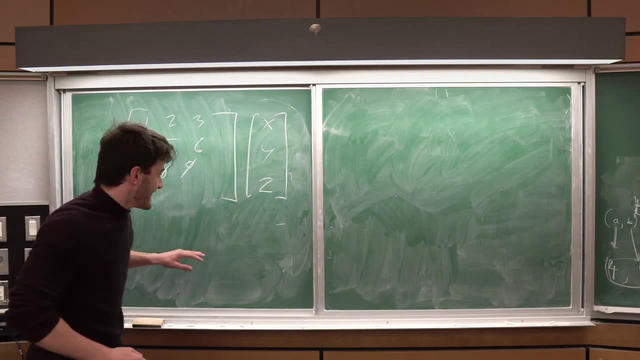 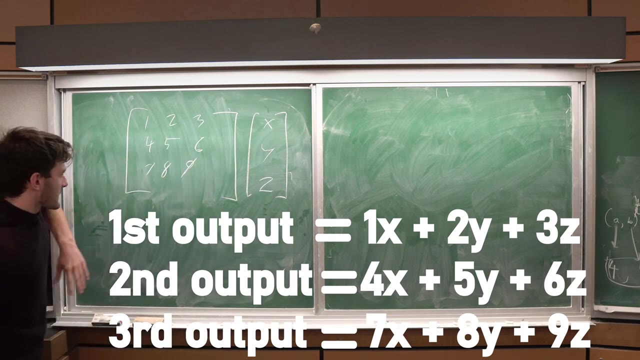 You can just put the coefficients in the actual function notation And so we do that by like. So what this says, What this says, that took me forever to understand. This is just a function. It's just a function. It takes in these, this thing. This is the argument. This is the argument and this is the function. 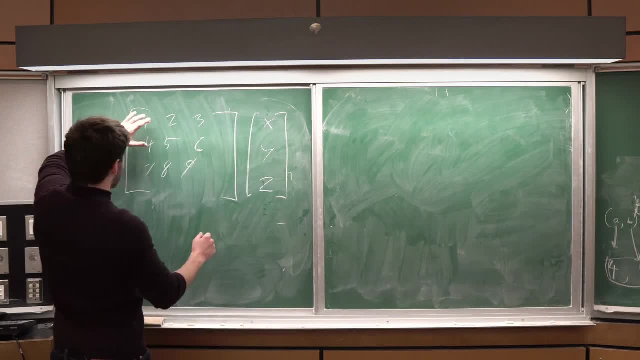 This says: take this right, XYZ. take X multiply by 1. take Y multiply by 2. take Z multiply by 3. Same thing for this row: take 4 multiply by Y. take 5 multiply by our shit. No, take 4 multiply by X, All right. take 5 multiply by Y. take 6 multiply by Z. and we just invented this. we invented this notation, this way of multiplying it. 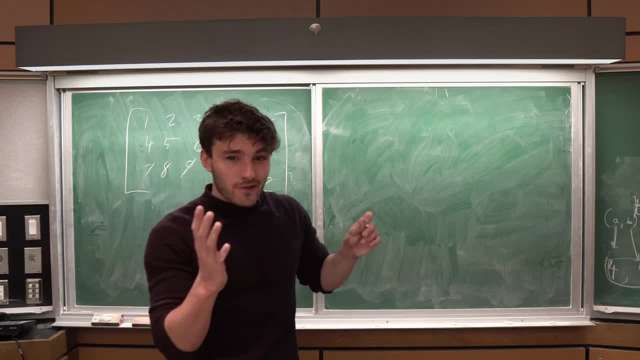 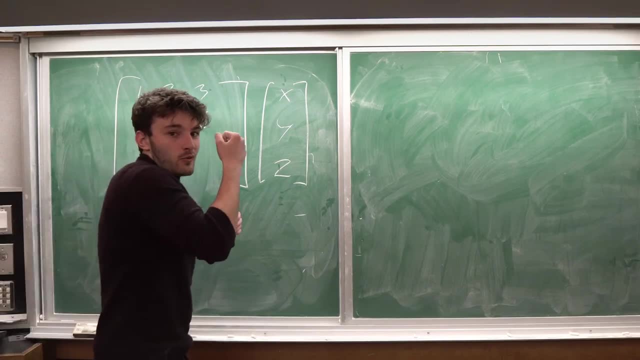 It's just a way of doing it. I mean, come up with your own way of trying to take a vector as an input and have a vector as an output. Just see how you can do it. There's a ton of ways to notify it. This is just one we've come up with, but it's just an arbitrary way of writing it down. 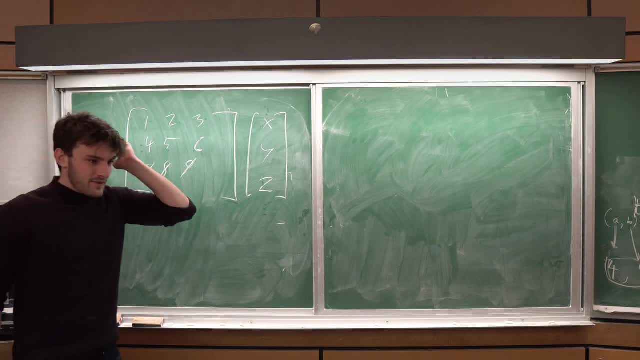 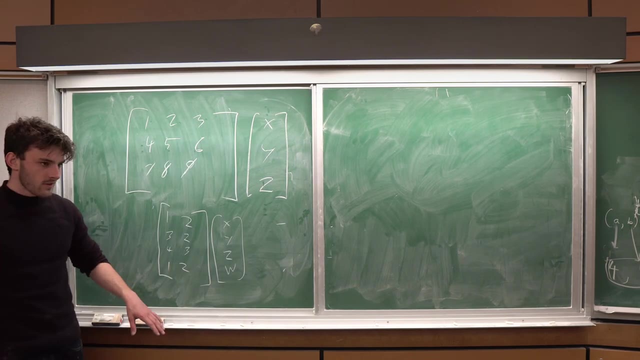 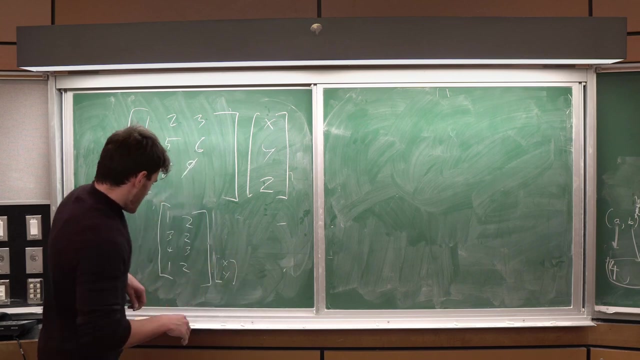 And so this is a function, you see, a matrix, think function, multidimensional in, Multidimensional out, and then I don't give you square, so you could have, You know, you can have it like. So this one, this one would take. So this one would take two dimensional input, two dimensional vector you fired into the function and it outputs a four dimensional vector. 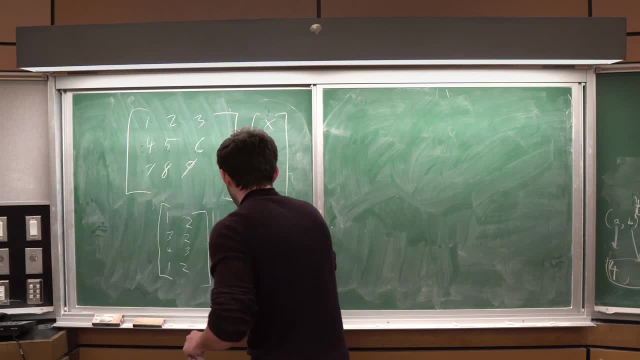 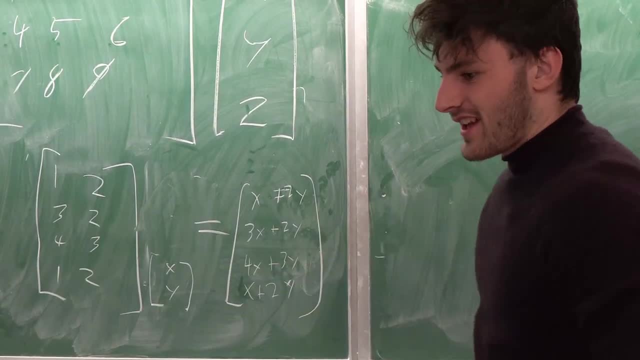 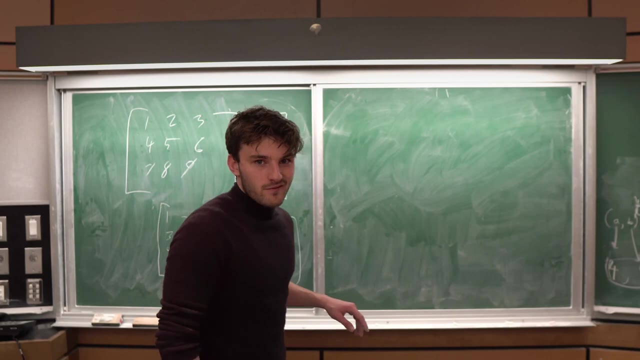 Because it has. it has four different things, so it'll have like. So this is a four dimensional vector from a two-dimensional vector and you can reverse it. you could have a four dimensional vector come in, Two-dimensional vector come out. you can have like a thirty seven thousand four hundred ninety two sized vector come in. 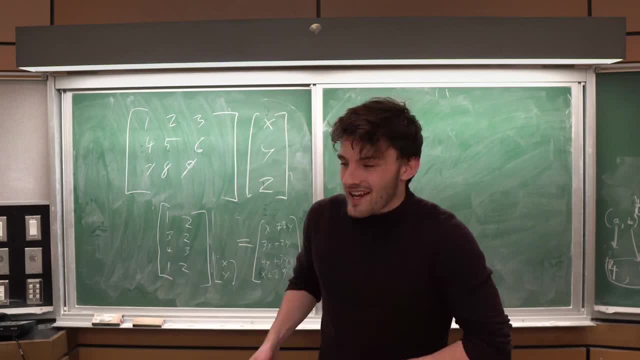 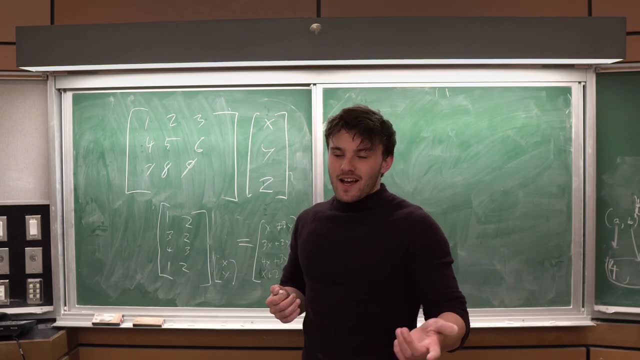 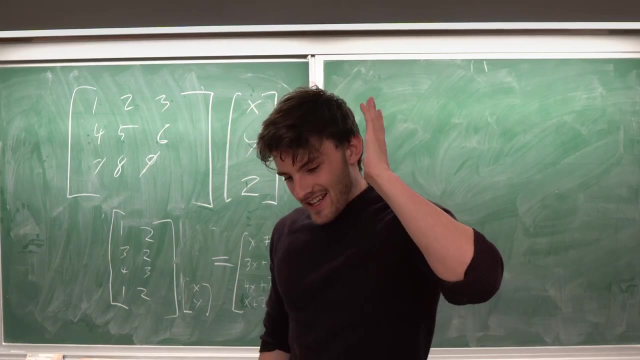 and like a 49,000 vector come out. you get crazy with it, and The study of linear algebra is just a study of these functions. So there's a bunch of stuff you can do. It gets quirky. There's a bunch of different eigenvalues, eigenvectors. 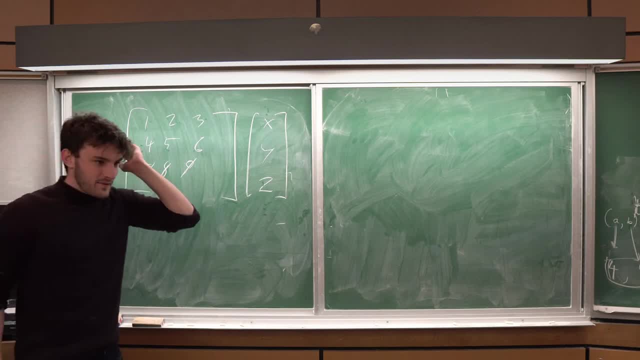 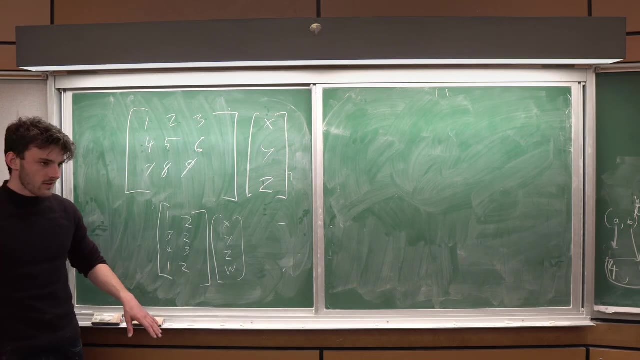 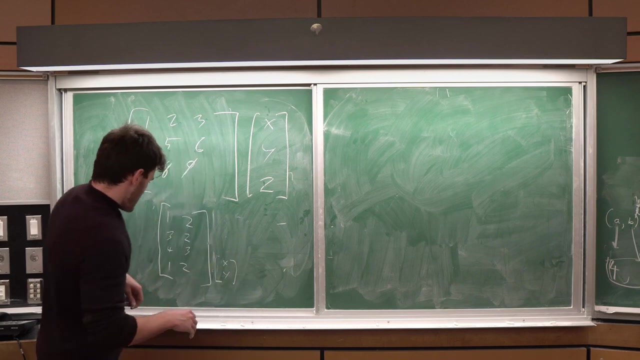 And so this is a function, you see, a matrix, think function, multidimensional in, multidimensional out, and then I don't give you square, so you could have, You know, you can have it like. So this one, this one would take. So this one would take two dimensional input to dimensional vector you fired into the function and it outputs a four dimensional vector. 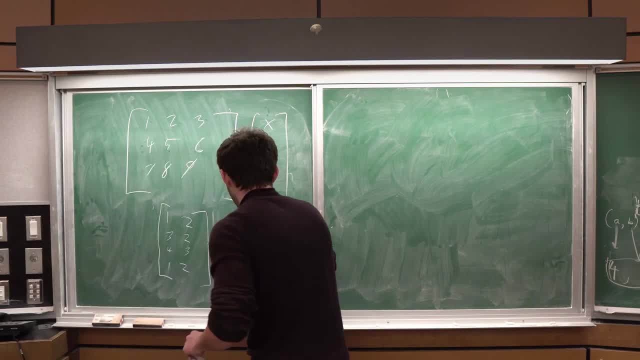 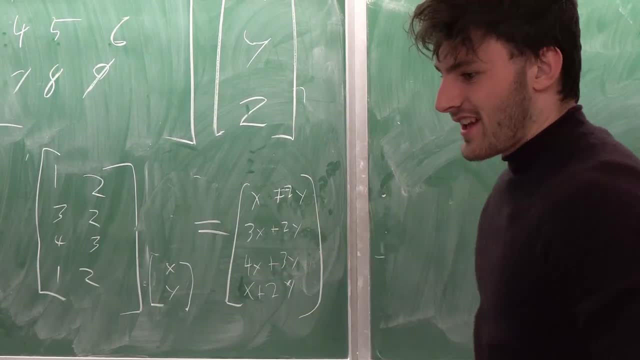 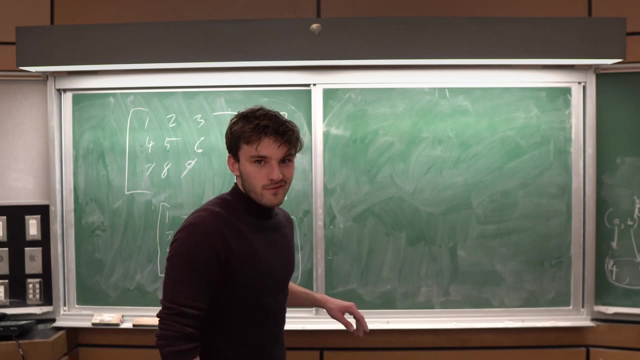 Because it has. it has four different things, so it'll have like: So this is a four dimensional vector from a two dimensional vector and you can reverse it. you could have a four dimensional vector come in, Two-dimensional vector come out. you can have like a 37,000. 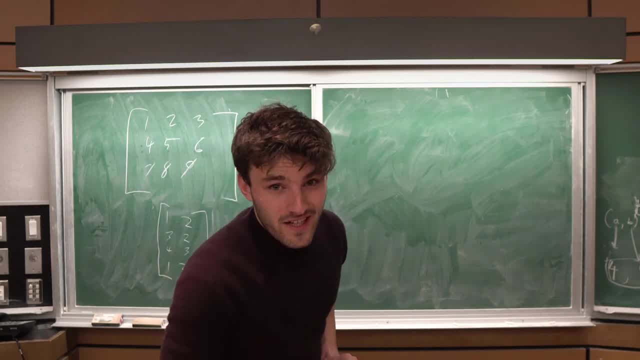 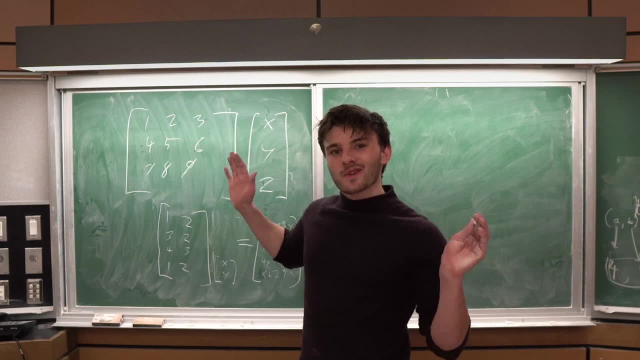 492-sized vector come in and like a 49,000 vector come out, you get crazy with it, And the study of linear algebra is just a study of these functions. So there's a bunch of stuff you can do. It gets quirky and there's a bunch of different. 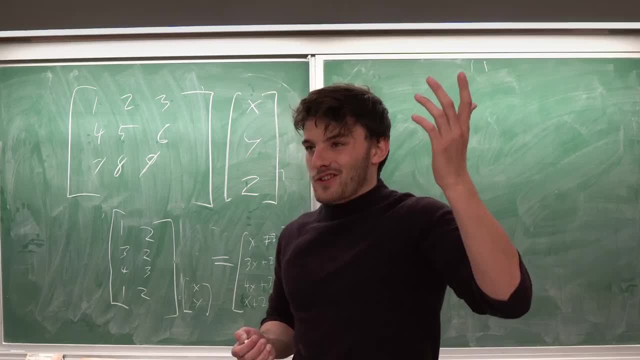 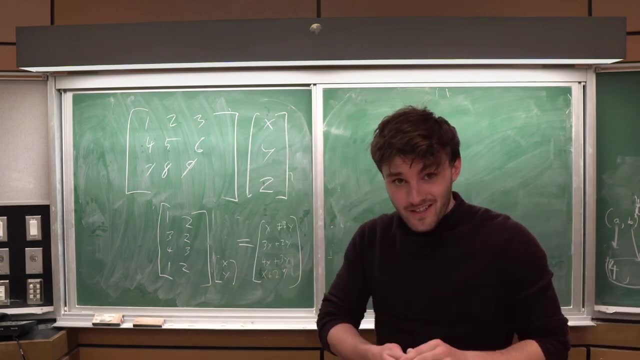 eigenvalues, eigenvectors, Like determinants. I hate determinants. Determinants are my mortal enemy. Not a fan of determinants, but you get the point. But linear algebra: when you look at linear algebra, it's just a study of linear multidimensional functions. 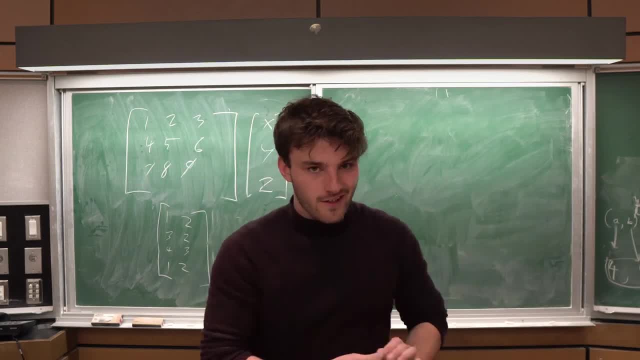 You take in a vector, you linearly do something to it and you fire another vector. I was intending that to be like two minutes long, but this is gonna be a pain in the ass to edit. It needed to be said though. 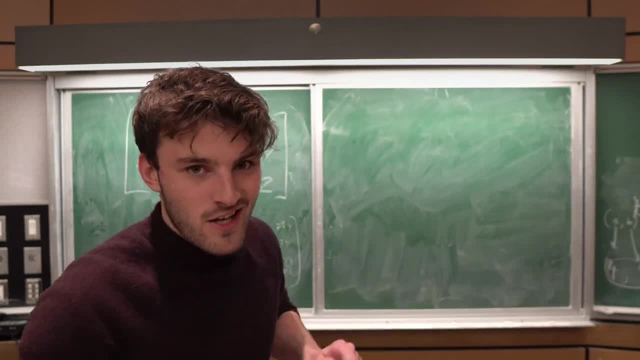 I'm gonna do a whole series on linear algebra so if this got confusing, I'm gonna try to do it a little bit better in the future. But when you see matrices, what I really want you to understand from this, the one main thing I wanna get across- 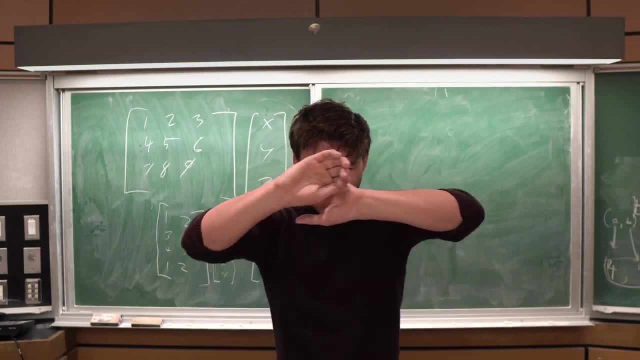 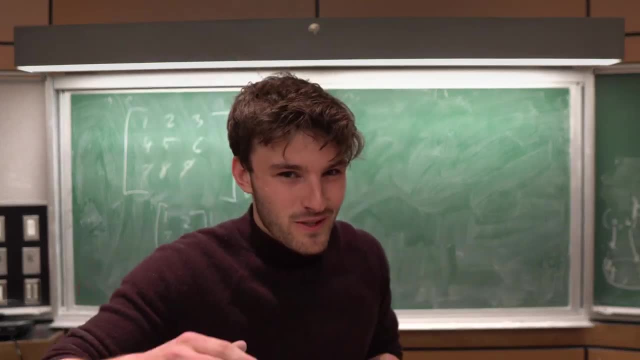 is when you see a matrix, it's a function. See a matrix as a function, and that should clear up a lot of stuff It did for me anyway. All right, maybe I do an outro, maybe I don't. If I don't do an outro, I love you guys. 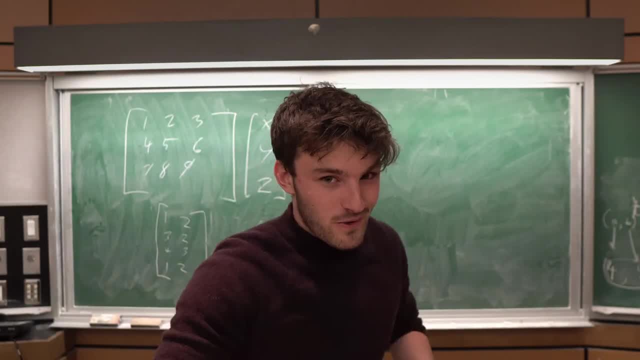 Take it easy and Godspeed. I will see you in the next one, which is tomorrow. Boy, do I have a lot to edit tonight. holy cow, Bye.